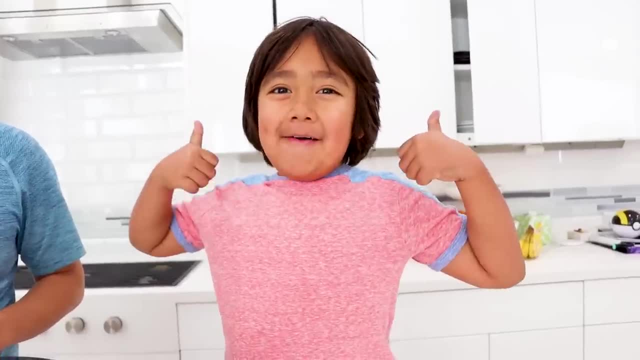 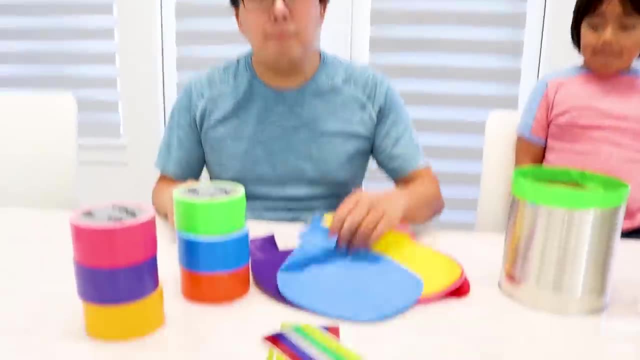 That's a great idea, Ryan. I'll help you, Thank you. Okay, guys, we gathered a bunch of other things that we need to make the drums Alright, so we gathered balloons- very colorful- and a lot of different colored duct tapes and stickers to decorate the drums. 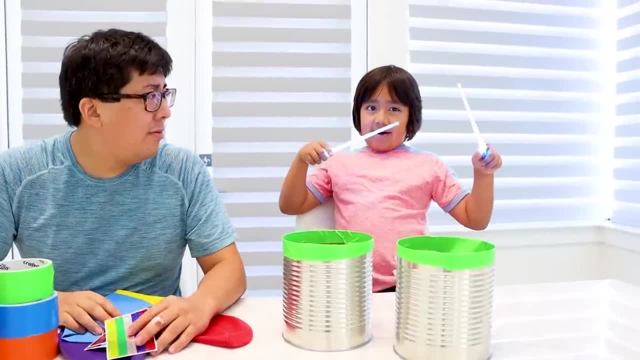 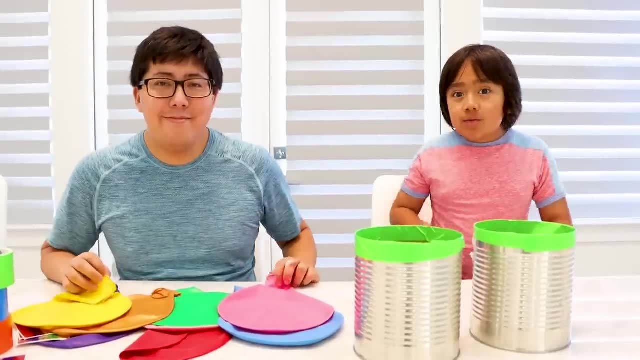 Yeah, And we also got light up chalk, Light up chopsticks, So we can use it as the drumsticks. First, we're going to use the balloons to cover the drums. That's right, Ryan, What color of the balloons do you want? 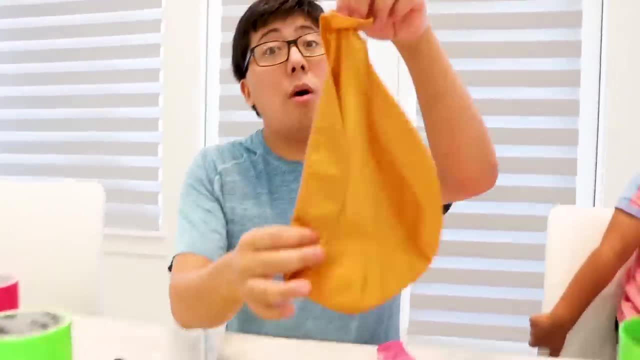 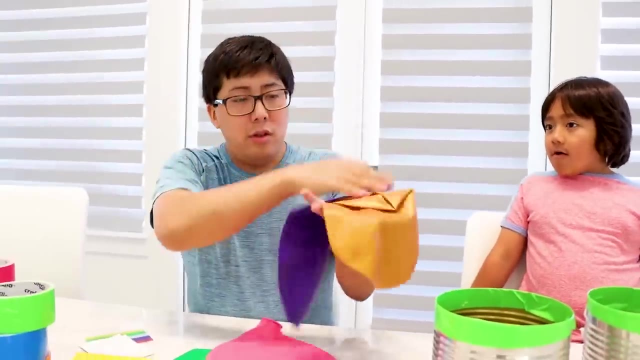 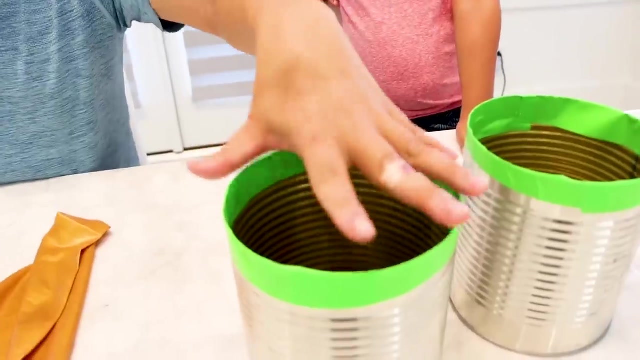 So many colors. I want gold- Golden, it is Alright. what's the next color? I want purple- Purple, it is Alright. so we chose these two colors. Now you have to cut out the balloons So it will fit over this container. 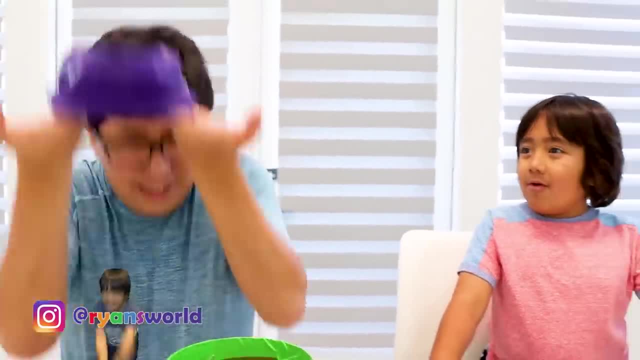 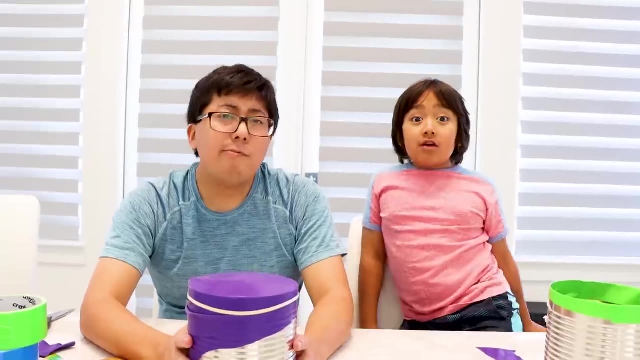 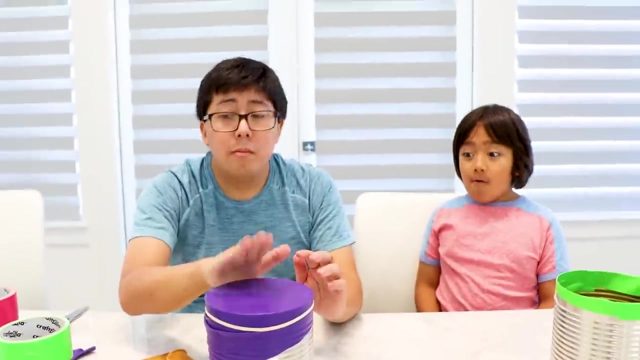 This looks like a swimming head cap, right, Yeah, Put it over here. You can also use rubber bands to hold the balloon in place. Now it looks like a drum, And now for the other drum. Alright, this is a special one, It's golden. 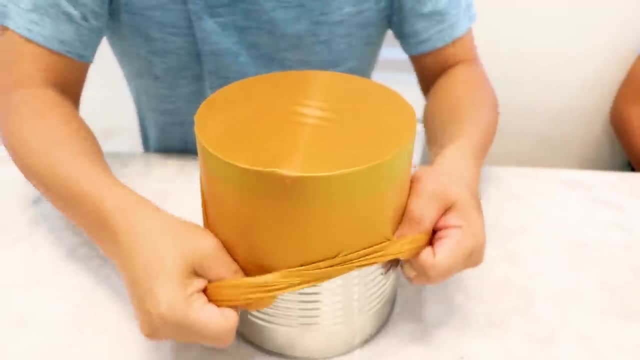 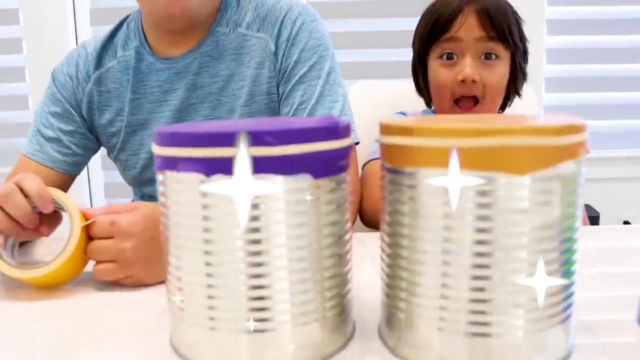 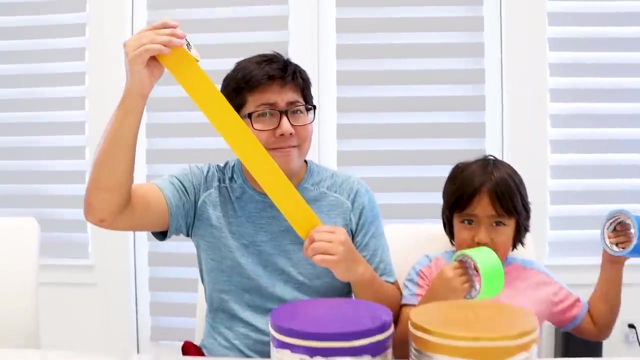 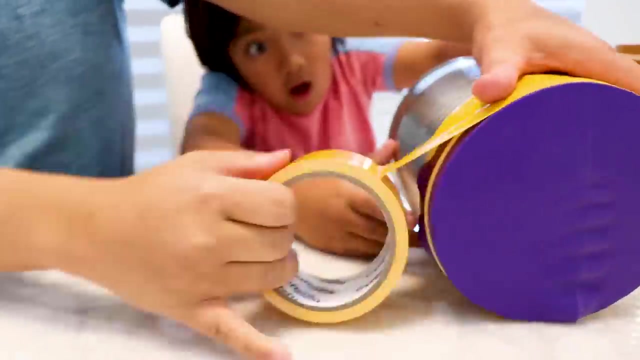 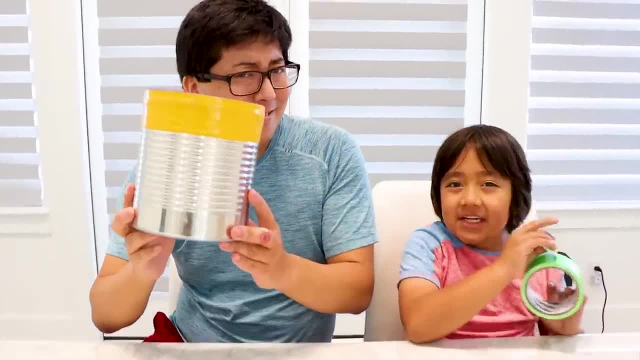 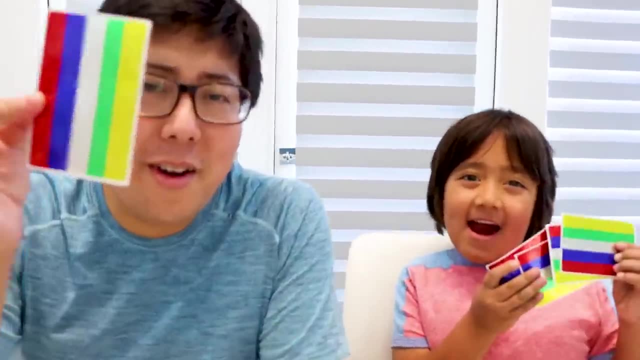 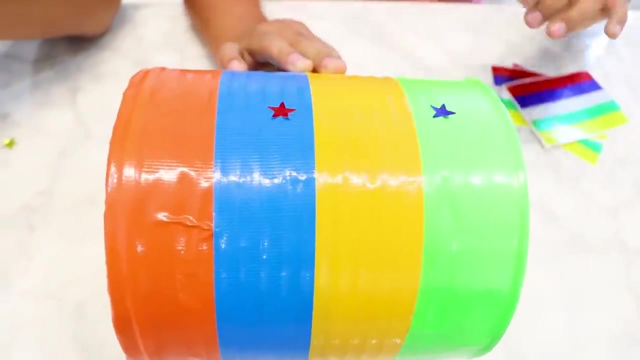 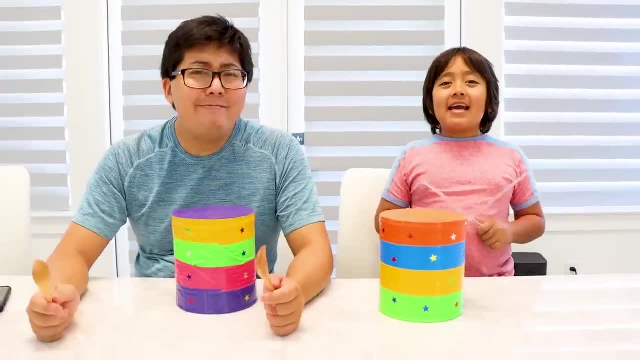 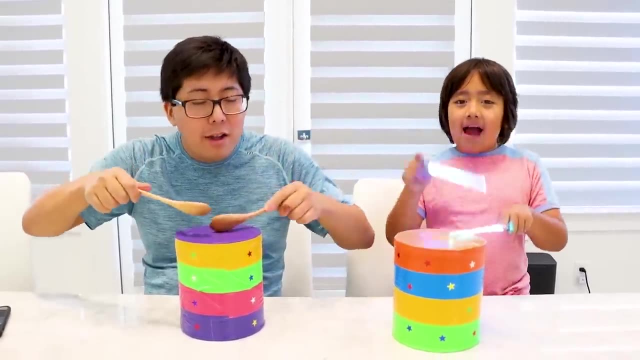 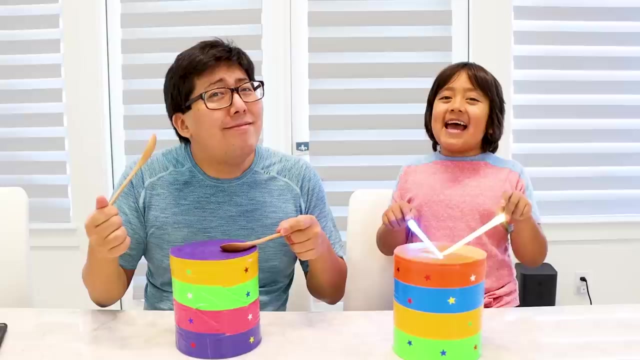 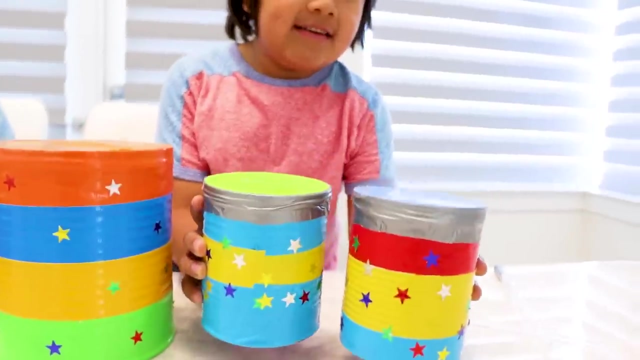 And yellow. Okay, guys, it's done. Let's jam. I hit the music. Let's build a robot. It's going to be my best friend. I'm going to build a robot. Grab some tools and let's begin. You can also make a smaller version like this: 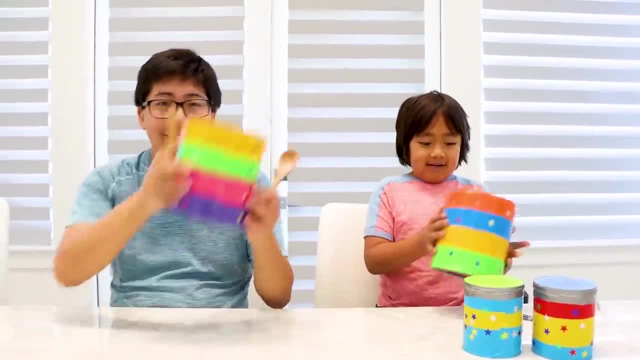 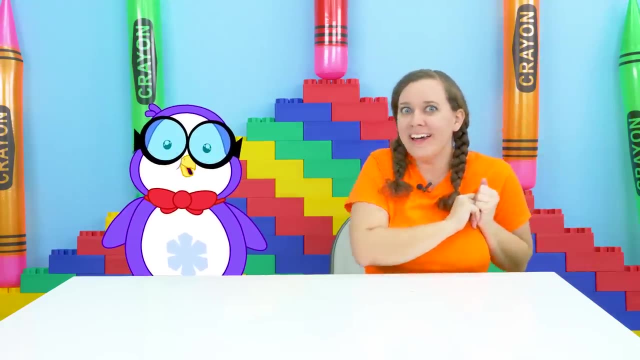 Come on, let's go And let's show Peck. Alright, let's go. Whoa, Oh, hey, Peck, Wait a second. If you're here, does that mean that Ryan sent us a new project? That's right. 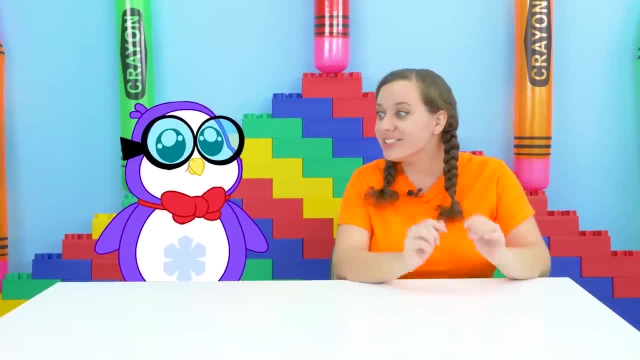 We got to make some musical instruments. Musical instruments, Oh man. that sounds like so much fun. I bet we could find things around the house to make them with. Let's find some things to rattle, make noise and do other fun stuff. 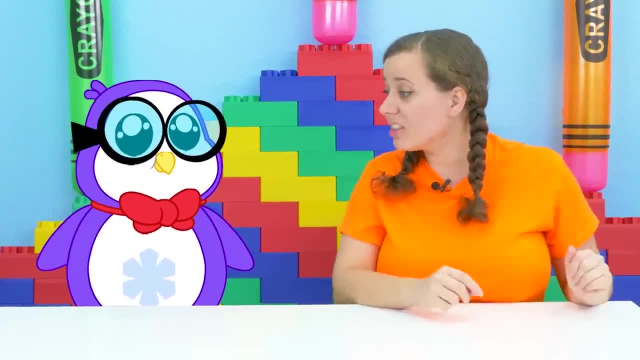 Yeah, no, that sounds great Peck, But we should. we should probably get going Like an instrument that uses strings, But we, we can go find these things. How about one that you have to blow into, which will make it a wind instrument? 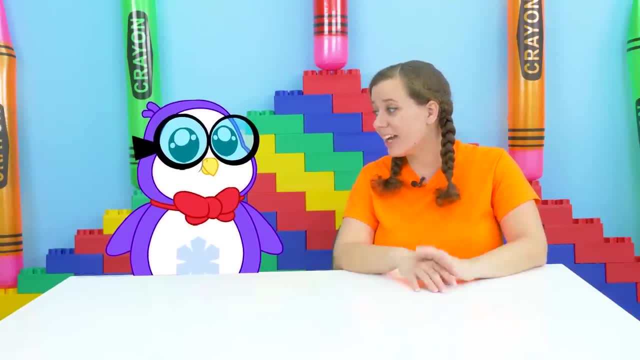 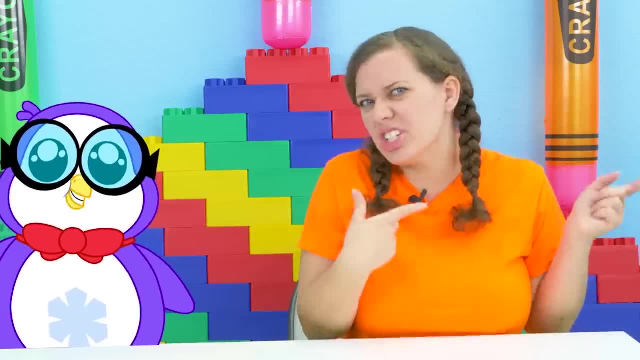 Peck, Peck, Peck, Peck, Peck. Oh man, what a hard day of work. It's time for my snack And it's Cheez-Its. Here we go, Cheez-Its all over my plate. 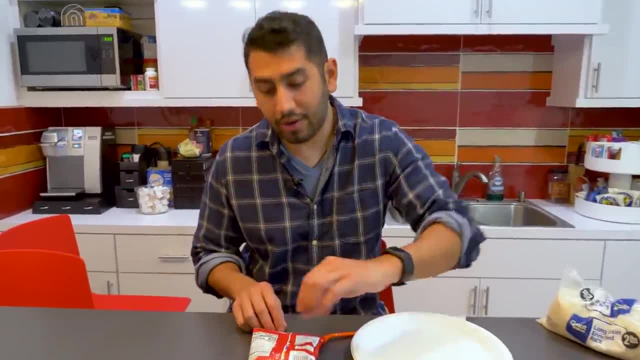 Now to eat this with my trusty spoon. Ooh a plate. Wait, what happened? Where's my Cheez-Its? I can't find it. Oh, Peck, Peck, Peck, Peck, Peck. 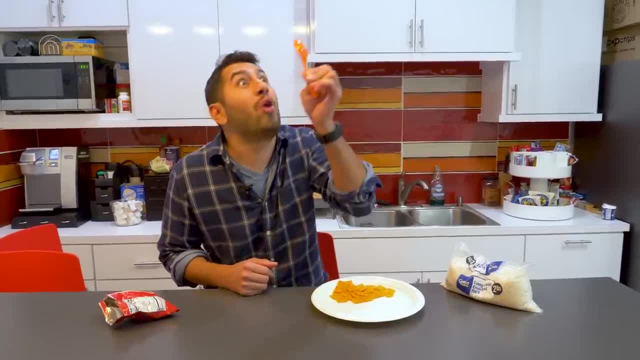 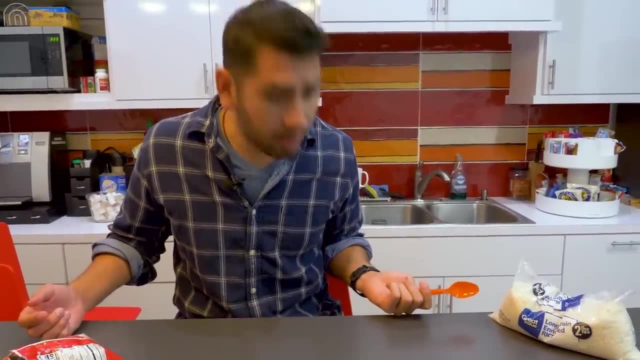 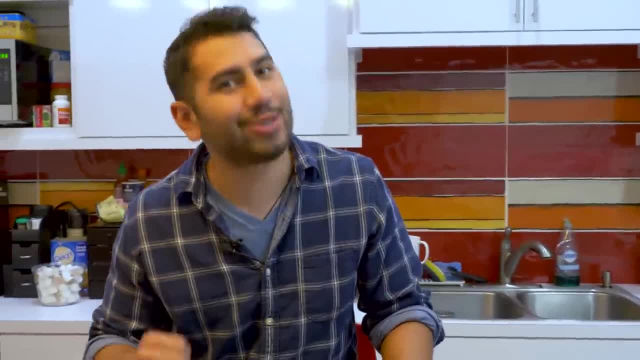 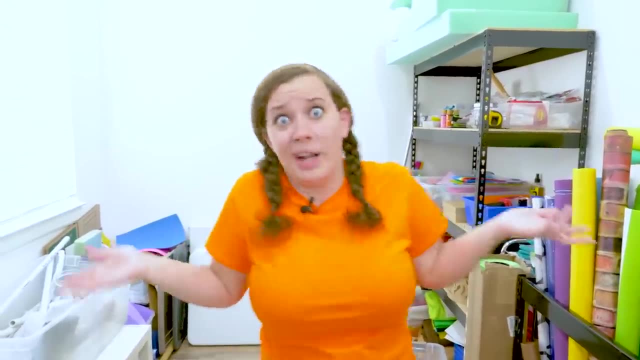 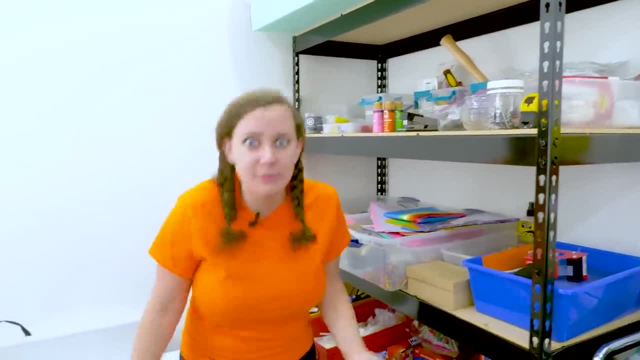 Oh no, Where did my spoon go? Oh well, At least I still have my long grain and rich rice. Wait, where'd my rice go? So, while Peck is doing whatever it is that he's doing, I know the perfect place to start. 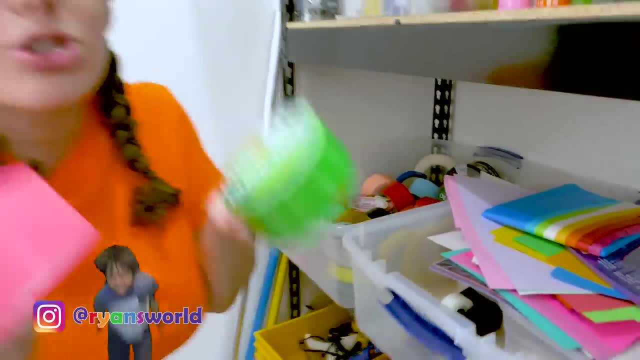 Come on, come on, come on. Okay, we have this whole shelf full of all sorts of arts and crafts and things like that. We need tape, and this is so bright and fun. Okay, maybe we could use some rubber bands. 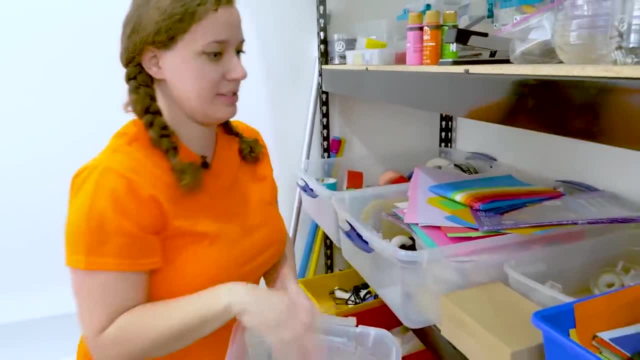 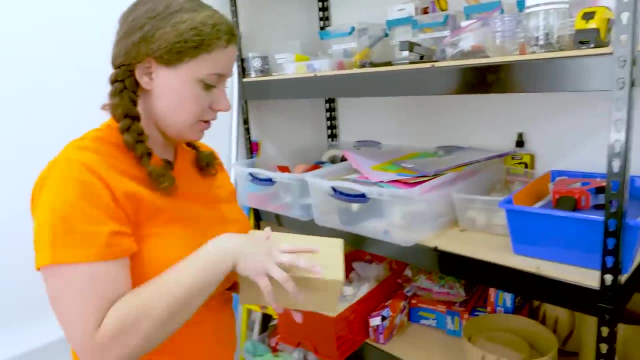 I mean, you can do anything with rubber bands. Let's get all of those, Definitely some colorful paper. I think that's a great idea. And, ooh, I wonder what's in here? Oh, look, how pretty and sparkly everything is. 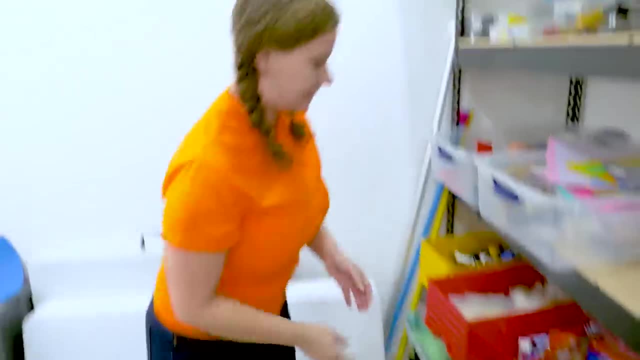 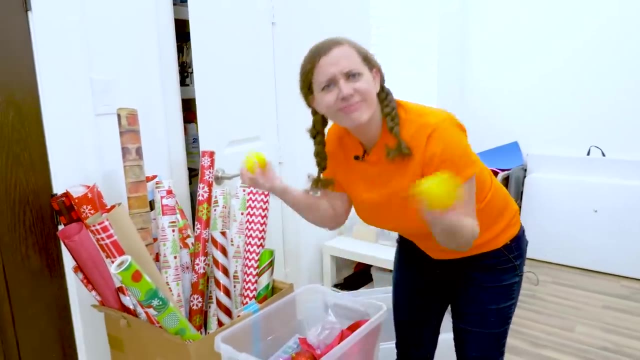 I don't know what we're gonna use this for, but we're definitely taking this with us. Jingle bells: That's pretty much an instrument already. Eggs: I don't think somebody put this back in the right spot, but I think we could use these too. 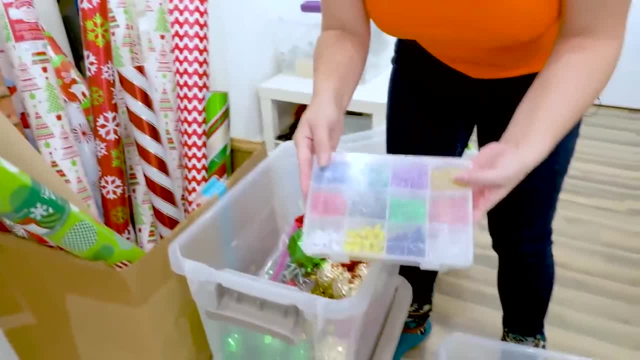 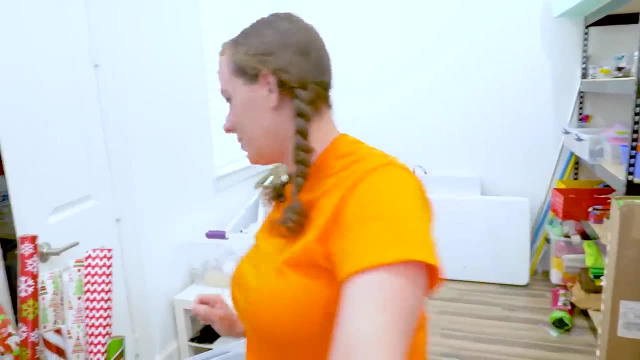 What else do we have? Wait, a second Thumbtacks. Well, they're bright and colorful. I think we can use those too. The last thing we need: I know what Wrapping paper. This is perfect, I have everything I need. 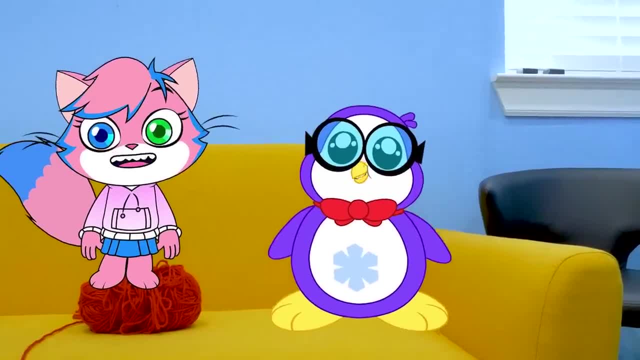 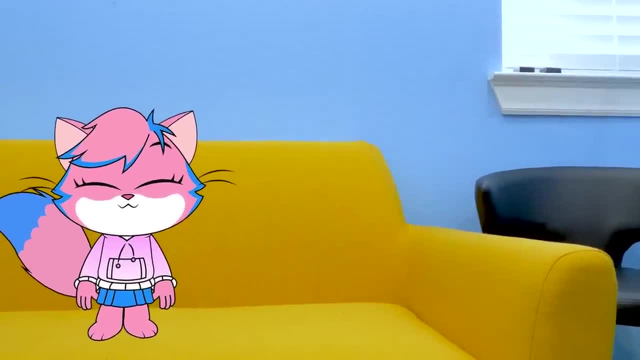 I wonder what Peck is doing. What do we have here? Yarn, I can use that That. Yeah, That's so silly. Just gonna borrow this toilet paper roll And there we go. Yeah, Oh, hey, Peck. 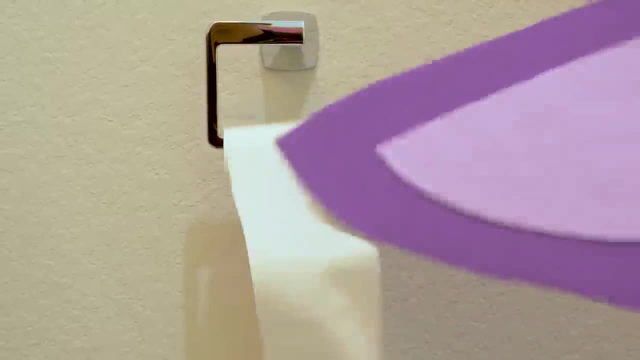 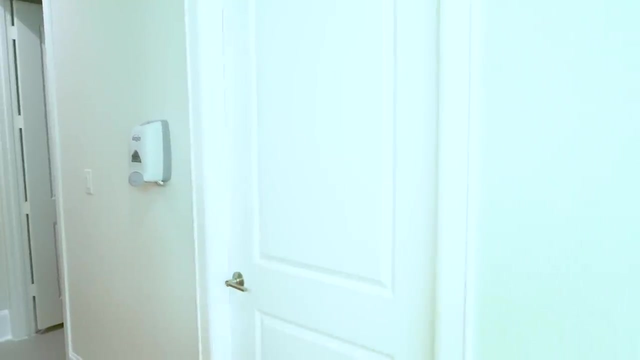 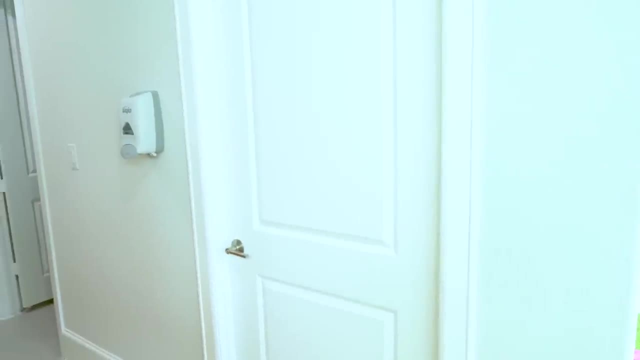 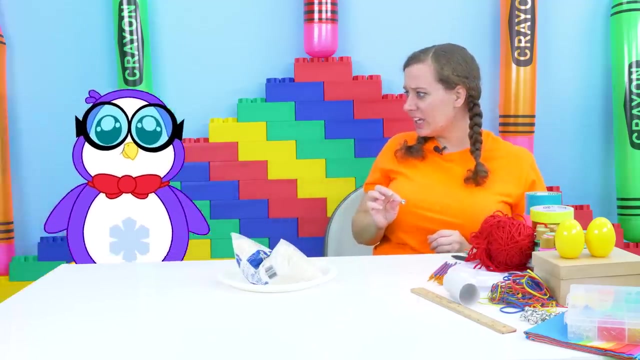 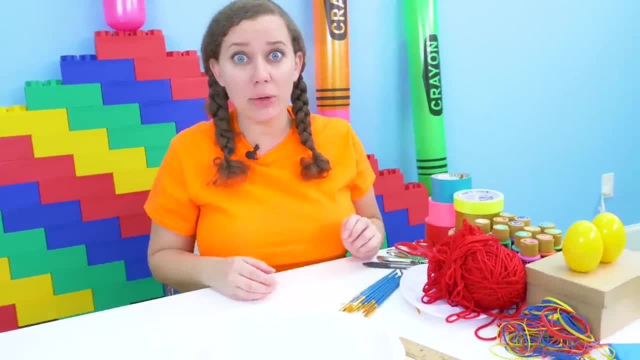 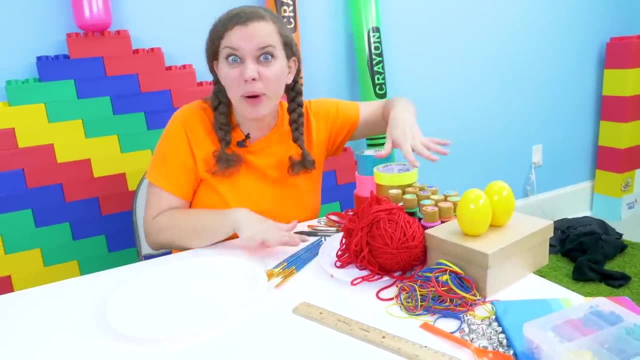 That's a great idea, Peck, And it looks like we have everything we need. For starters, we can use this plate to be the base, But it's kinda white and plain, so we can paint it- maybe some bright, pretty colors. 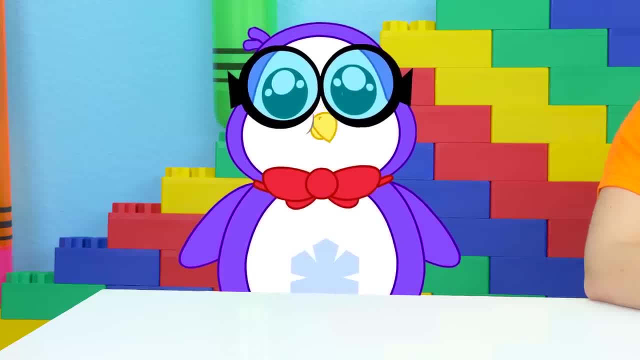 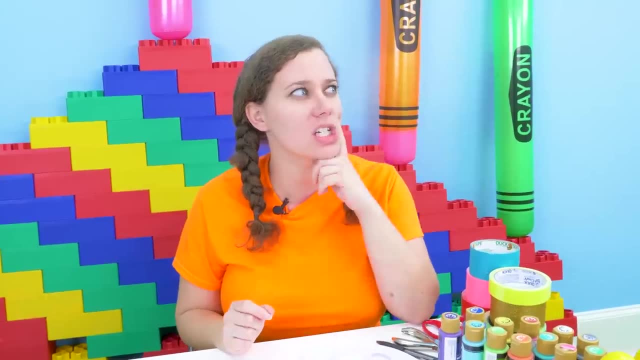 I don't know how that's gonna work, but I believe in you, Bree. Oh, I have the perfect idea. What is more colorful than a rainbow? So we need all the colors of the rainbow, which is ROYGBIV. 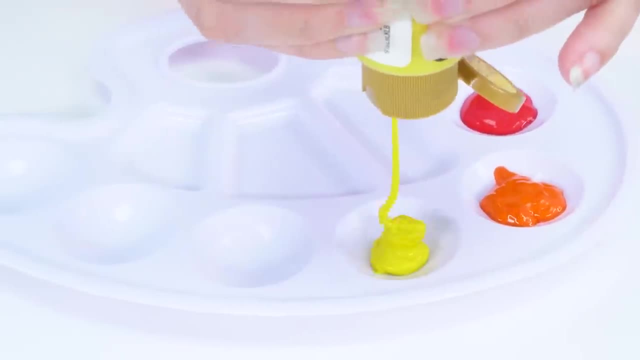 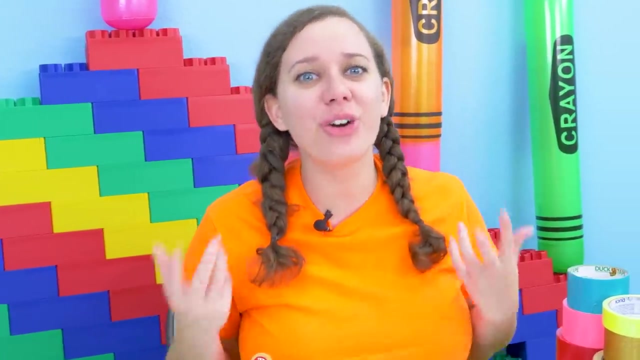 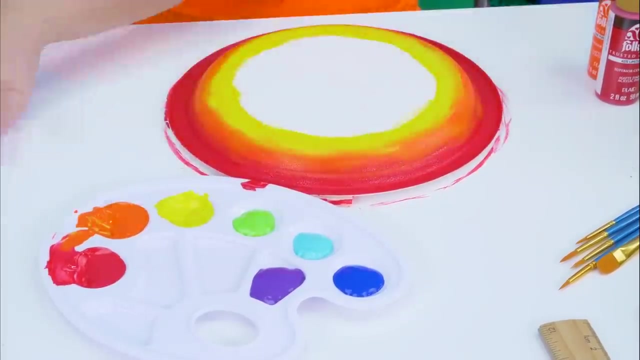 So it starts with red, and then orange, yellow, green, blue, indigo and Violet- Violet, of course. I kind of forgot your color pack, Sorry. Whoa, looks like a rainbow now, Cool. So the next thing we need to do is try to fold this up like a taco. 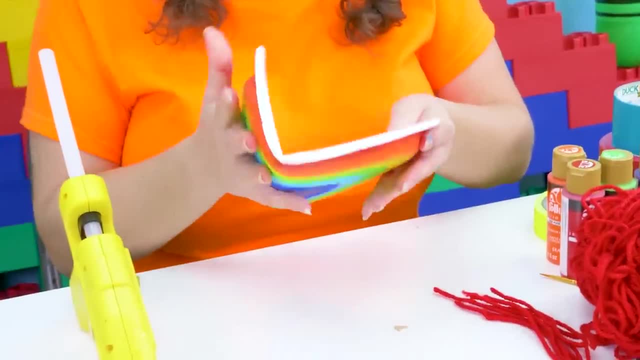 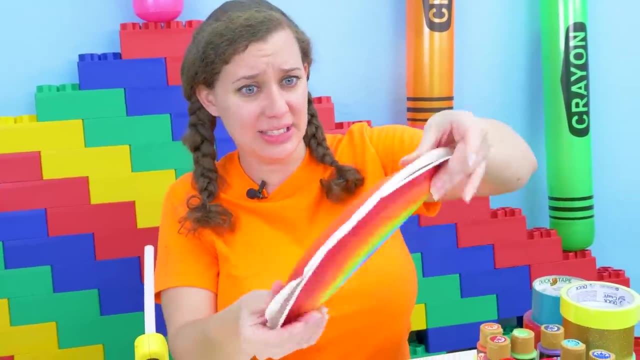 So we have only half a plate. We have a rainbow. Let's see if we can make it work. Look at that: We have a rainbow. Wow. Now I think we need to glue it together. All the glue- We need lots of glue for this, because this has got to hold tight. 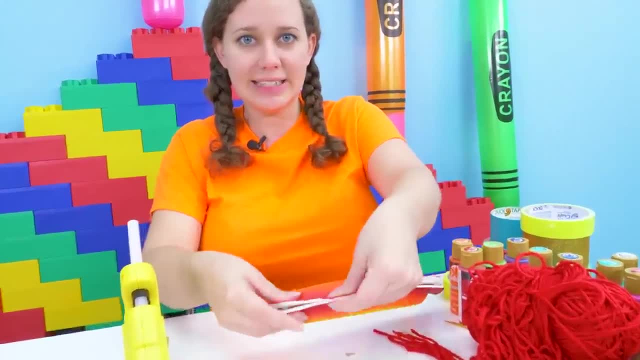 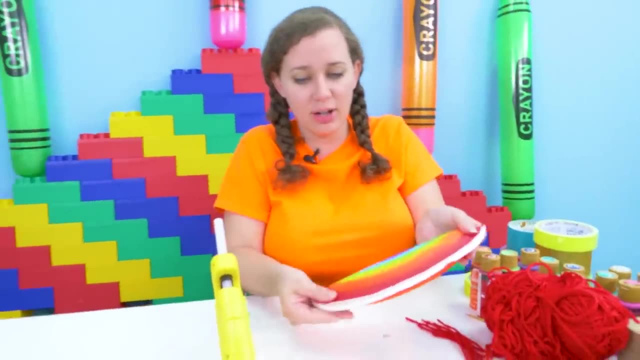 Three, two, one and we're smashing it together. Oop, it's a little hot. This is why you need an adult for help. okay, Because hot glue can get really hot. There we go. Look at that taco. 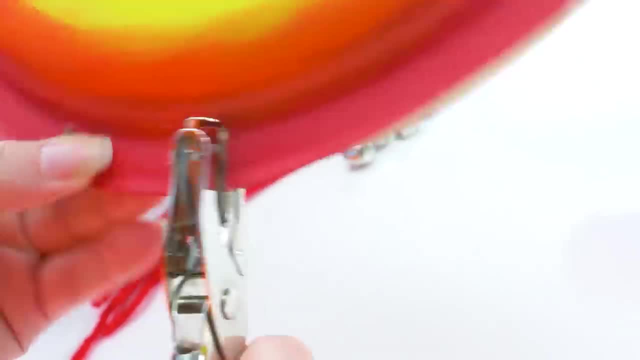 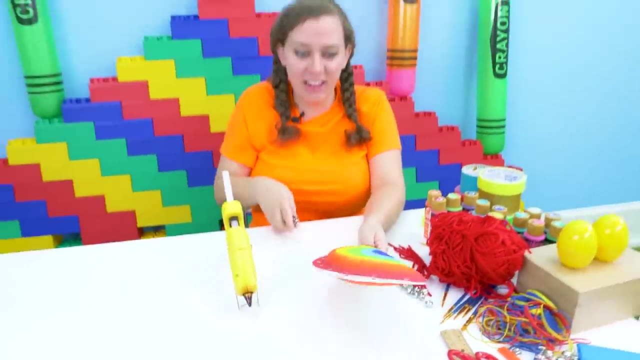 Nom, nom, nom. All right, hole puncher. We need one hole for every jingle bell And last one. That was a lot of work. Now we're ready for the jingle bells. We put each bell on a string. 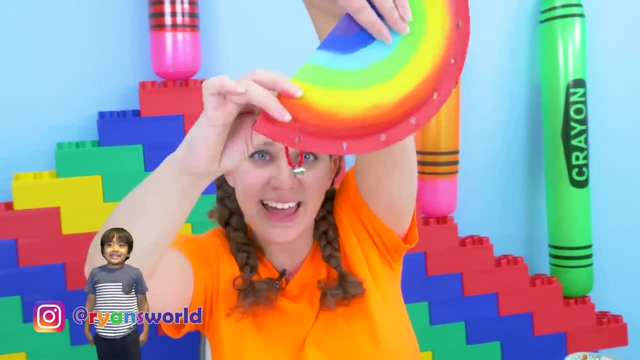 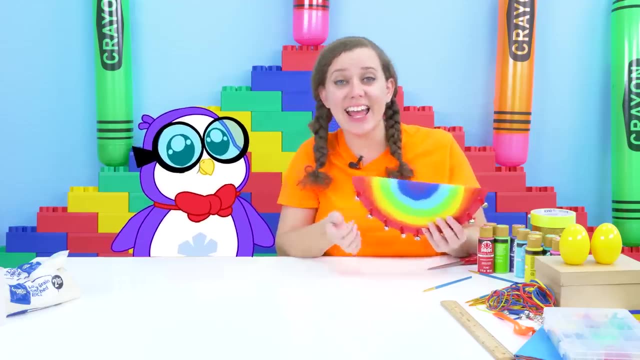 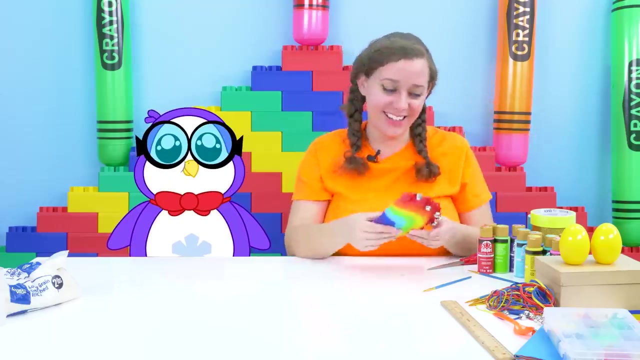 Now we're just going to take the string and tie it to each one of these little holes, like that Ta-da And done, Done. And once you have them all tied up, guess what? you have A tambourine. Cool, Now let's make some maracas, Yeah. 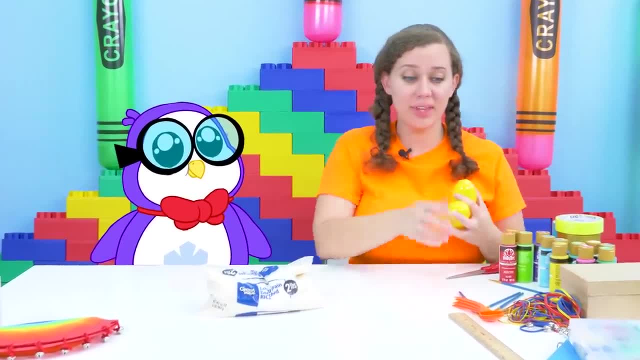 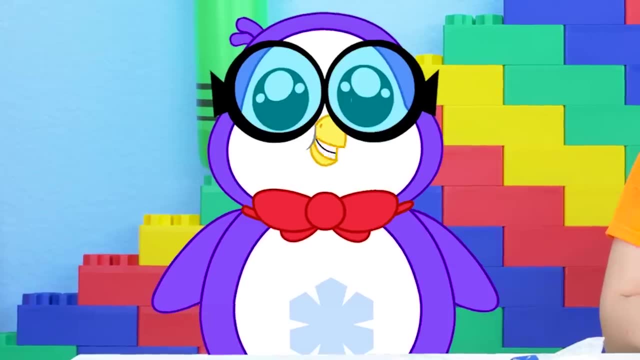 Okay, so for maracas, we can use these eggs that we found some spoons, and we can use your long grain enriched rice pack, Of course, The long grain enriched rice. So the first thing we're going to do is we're going to put some rice in these eggs. 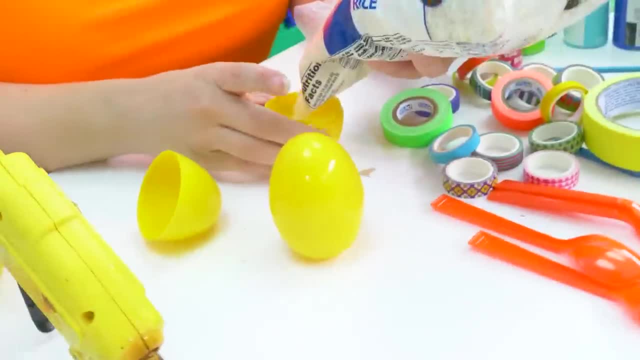 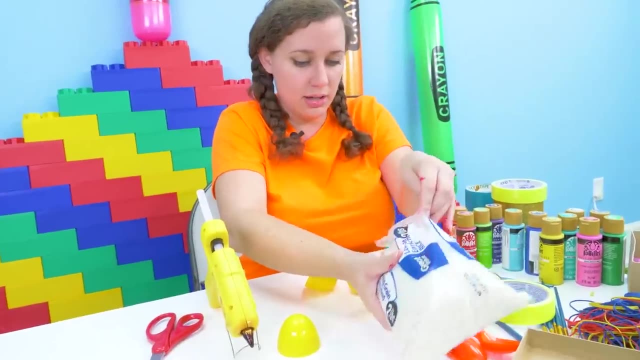 I think I'm going to make a mess, Okay, But it's okay, That's part of crafting. So we need some rice to make some noises. Ah, Okay, I'm making a lot of mess. There we go. Now we're going to put the lids on and see if it sounds. 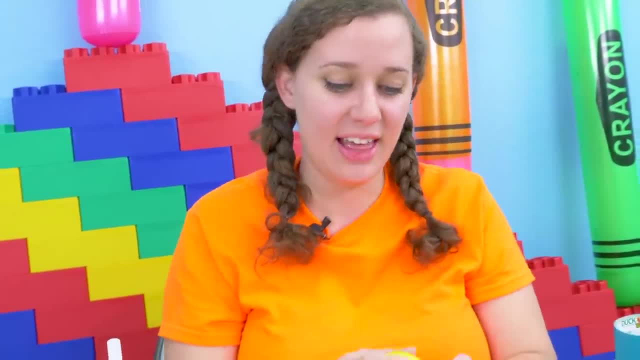 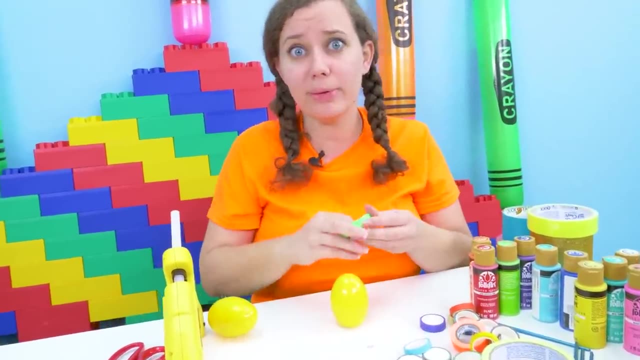 Oh, That's so cool. All right. number two: Now we need to make sure these don't open, so we don't get rice everywhere. So maybe we should use some tape, Whoa, Seal it up nice and tight. That ought to be good and sturdy. 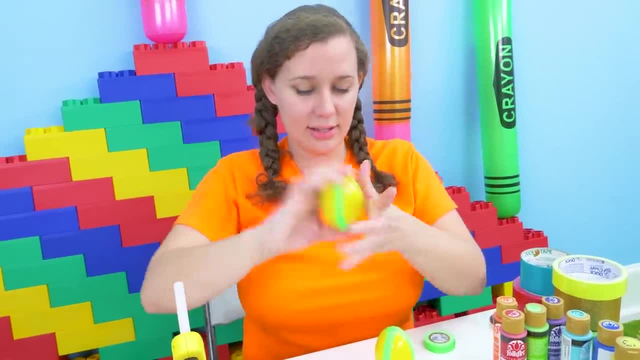 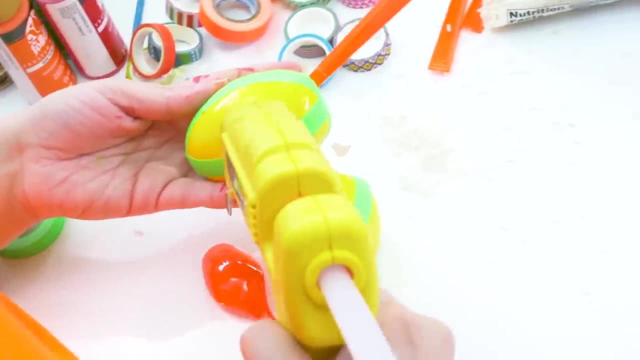 Sounds good to me, All right. So now we're going to glue the spoons like this to make a handle. You've got to be careful with the hot glue. And ooh, there we go. Handle number one, handle number two. 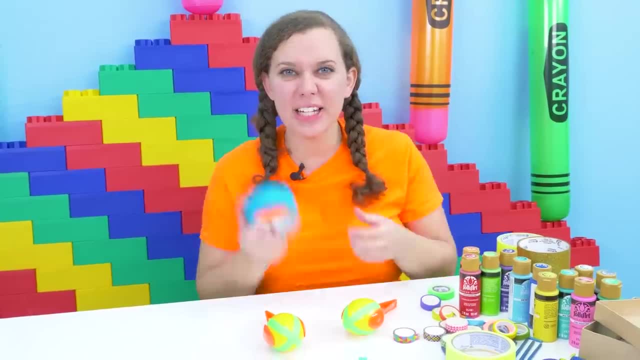 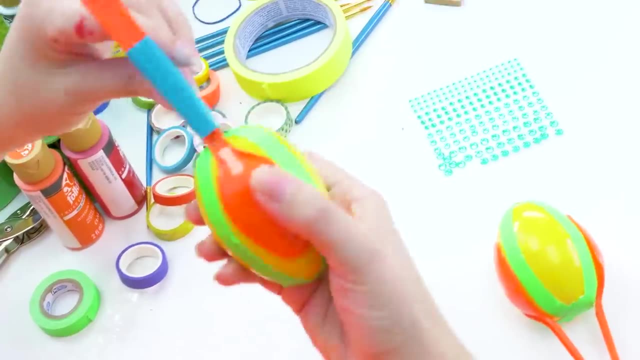 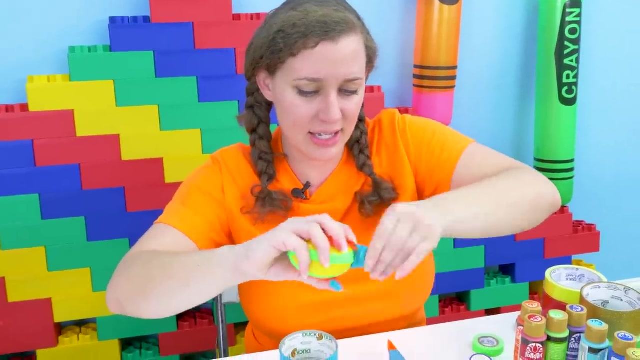 All right, There we go. Next we're going to tape it up and then decorate. All right, Taping, taping, taping, taping, taping, Tap, tap, tap. Ooh, Perfect, Last wrap and done with that. 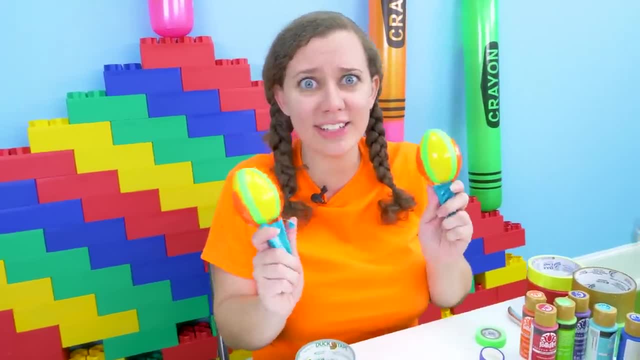 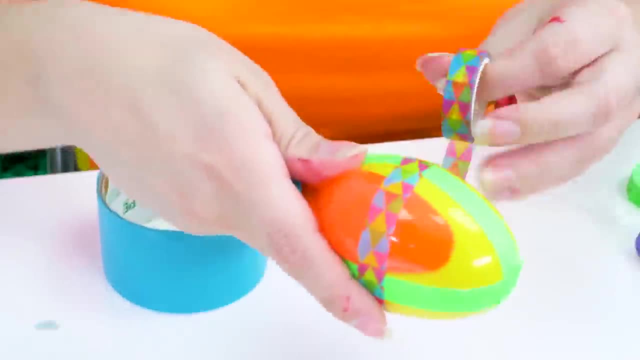 I think we could use some decorations, though I mean they have to be festive, right. Peck, Yeah, Time for the fun tape. Oh, it's so cute. Look at all those bright colors. Super festive, There we go. 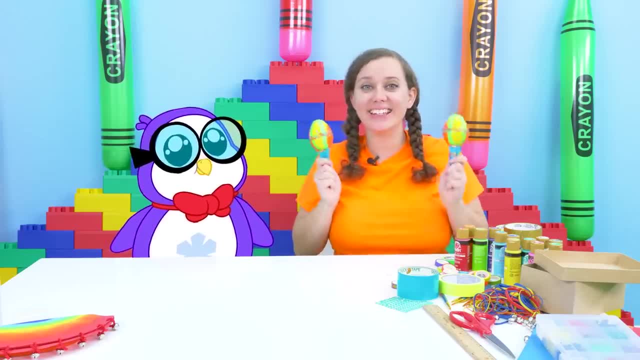 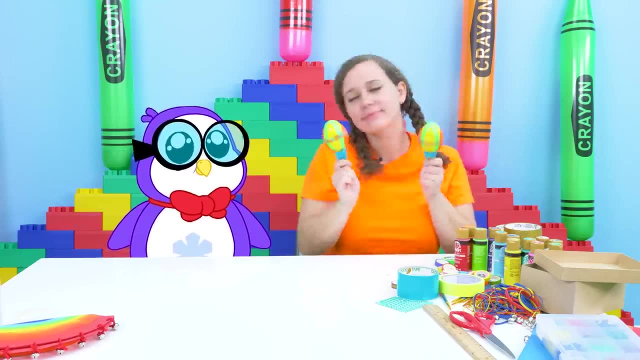 Ooh, maracas Spectacular. Yes, I mean, the festive tape is definitely what made the maracas, so listen to that, Okay. well, next we can use the toilet paper roll for something You know what Peck. 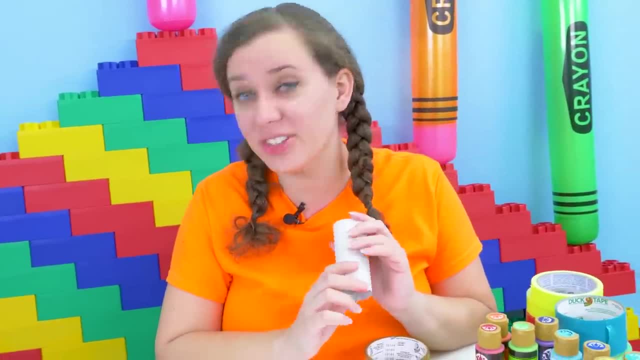 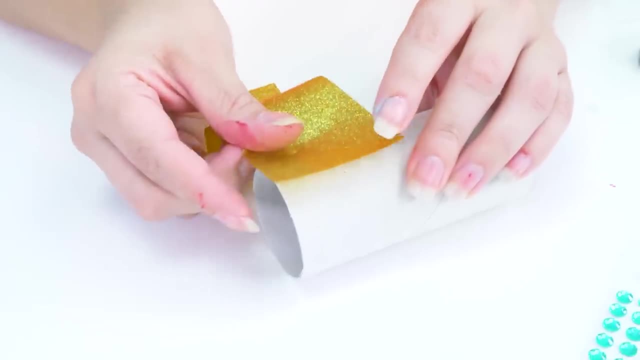 I actually have an idea for the toilet paper roll, but it's going to be a surprise, so you're just going to have to wait and see what it is. We're going to start with this super shiny, sparkly tape, Okay, so just because we don't want it to look like something that came from the bathroom. 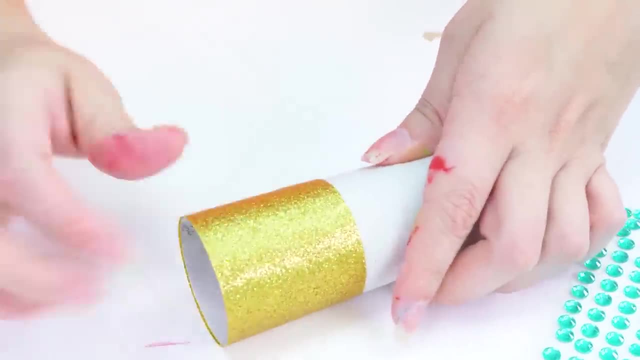 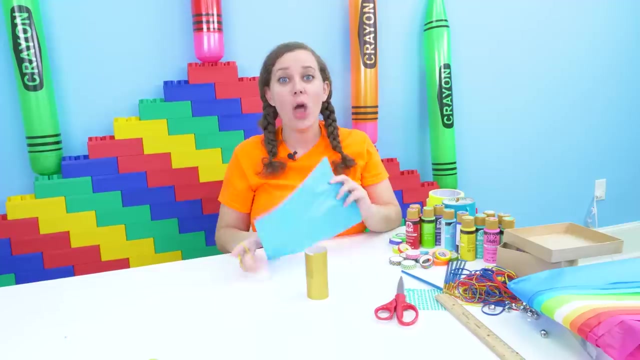 we're going to wrap it in this super shiny tape. Ooh, that's so pretty. All right, Let's cover this other end. There we go. We're going to take the tissue paper- crinkle, crinkle, crinkle- and put it on the edge of. 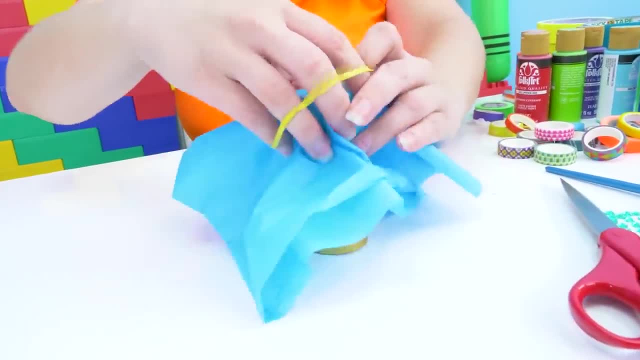 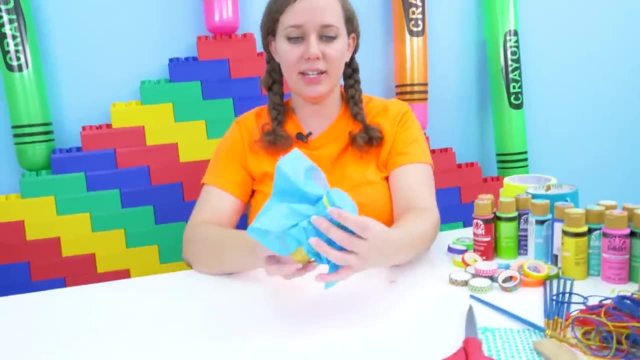 this with a rubber band: Squish, squish, Ready Dun dun. The science of rubber banding things together. Super technical. There you go. Well, now we can't really see our kazoo, so maybe we should trim this up some. 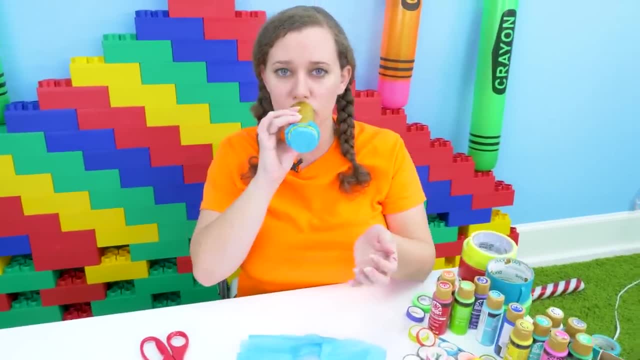 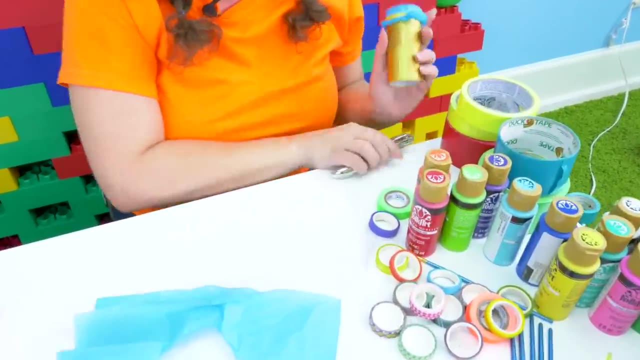 Oh, that looks so much better. Now we can actually see our kazoo Da-da-da-da, Oh, Da Da. We're catching a little bit of air here, so I think I have the perfect thing to help us out. 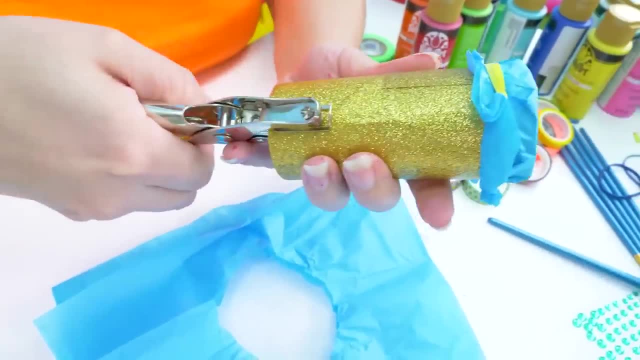 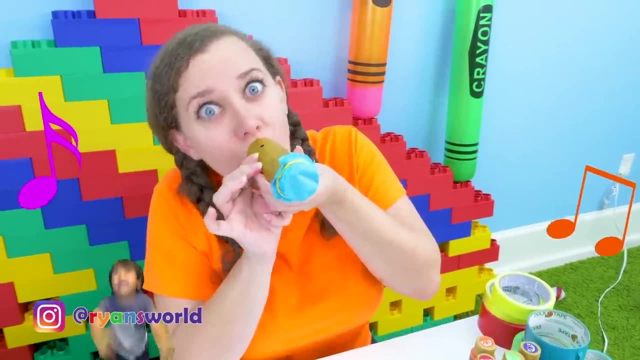 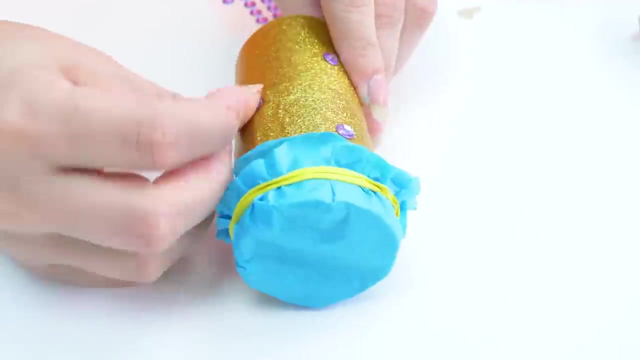 We just need to make a little air hole. Oops, backwards Bink. Let's see if that works. Da-da-da-da, Da-da-da-da, Da-da-da, Da-da-da. Oh, it works so good. Since this is already shiny- and we have these shiny jewels- why not just decorate it a little? 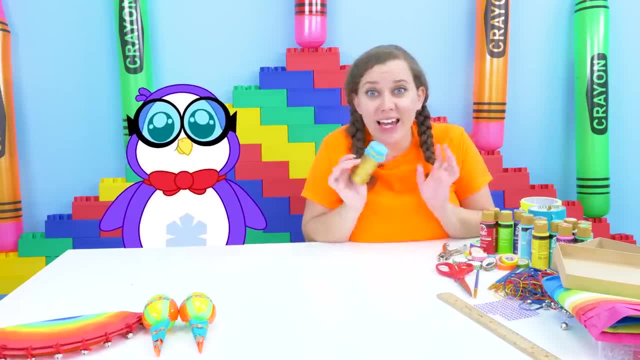 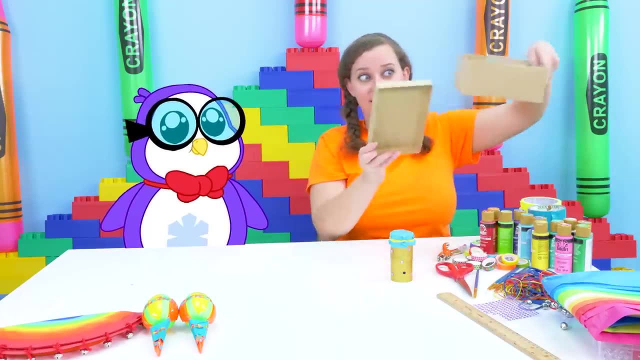 bit. You know, for some extra credit, We got all our jewels on Pack. what's next? The last one will be tricky: A guitar- Ooh, I have the perfect body for that guitar. What about this? That'll work. 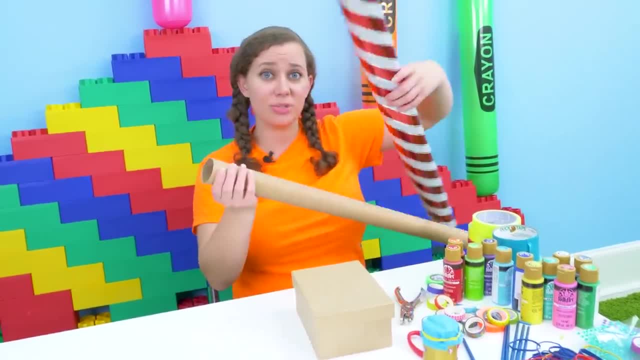 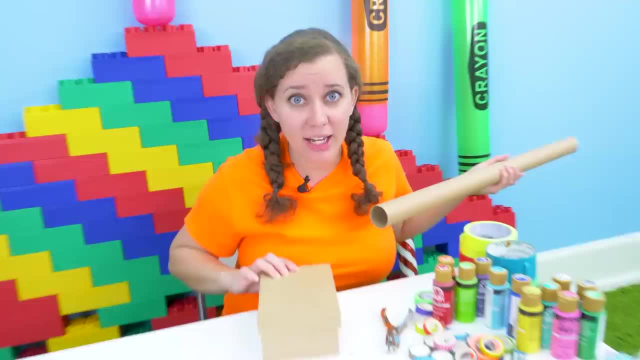 So we're going to start with the neck of the guitar, which we can actually use, the wrapping paper roll that we found. This is a little long, so we're definitely going to have to shorten it, And then we have our body, which is this box. 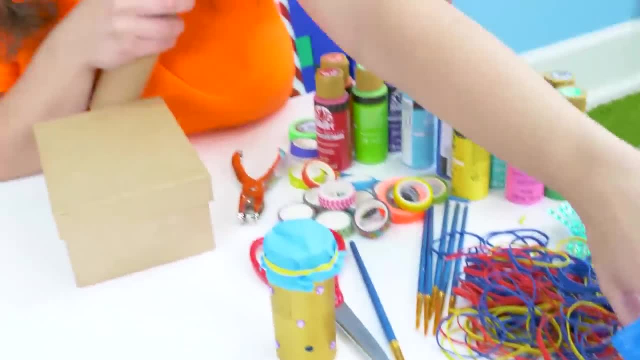 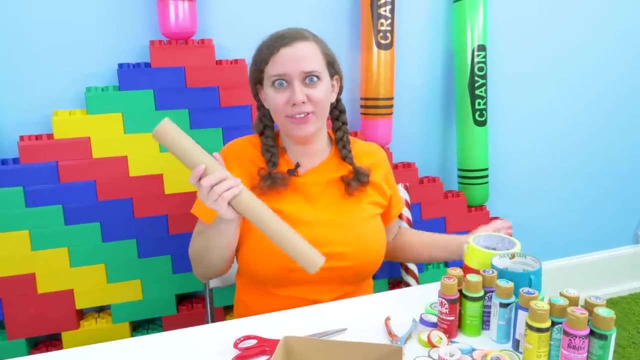 We have strings to pluck and play with, and I think we even have little tuning knobs that we can use. Yeah, Hi-ya, Ah, perfect length. So now we just need to cut a hole so we can stick this guy through it. 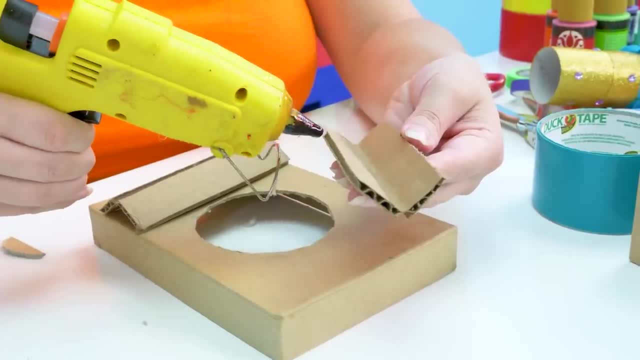 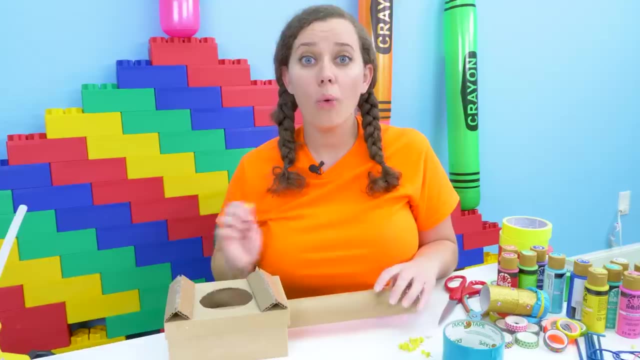 Ding, Perfect hole. So we're going to use these pieces of cardboard as string holders to hold our strings in place. Ooh, All right. While we're waiting for the glue to dry, right here, which this is what's going to hold our 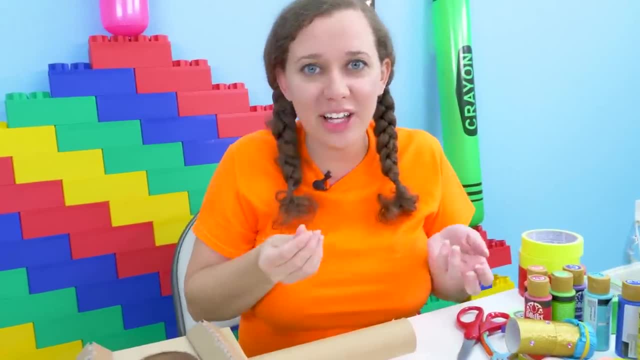 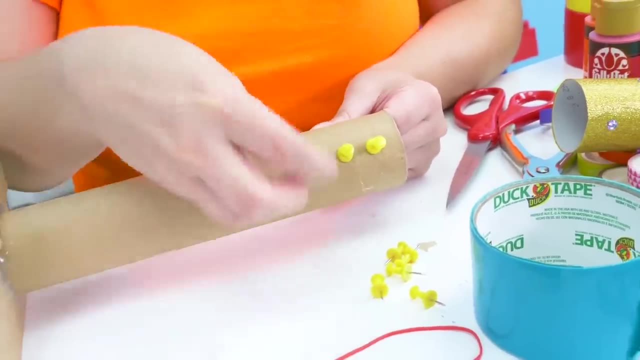 strings in place. let's put some little tuning knobs. Of course they're not going to work, but I think it'll really help it look like a guitar. So we need six of them: total One, two, three, Awesome. 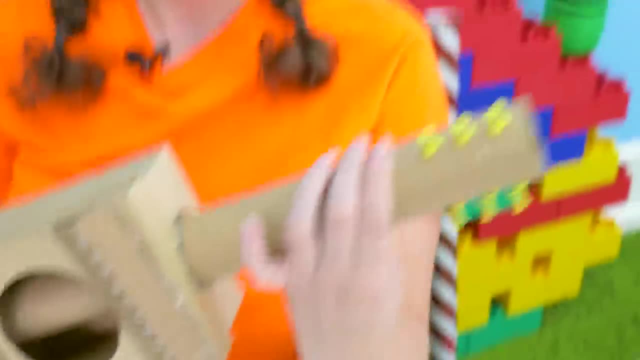 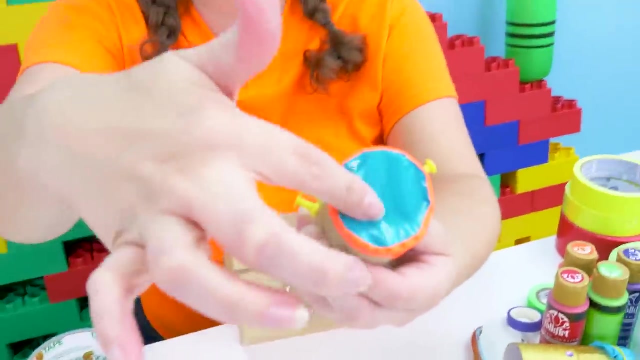 And then the other side. There we go That way. when it goes out of tune, you can just tune it up, Just like that. So we sealed up the ends. That way you can't get poked by any of the thumbtacks. 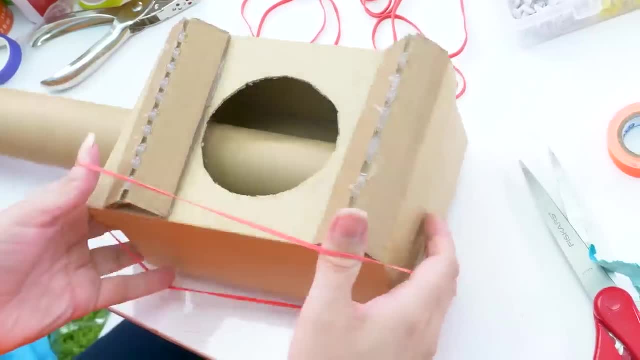 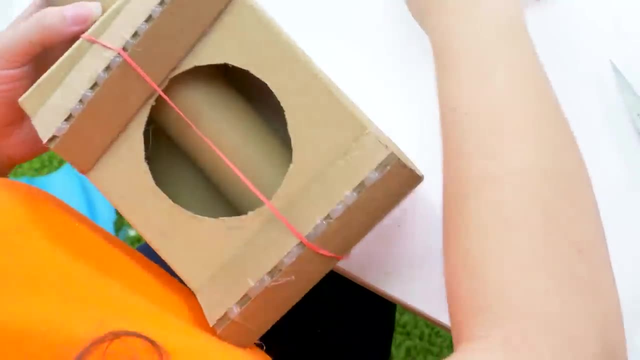 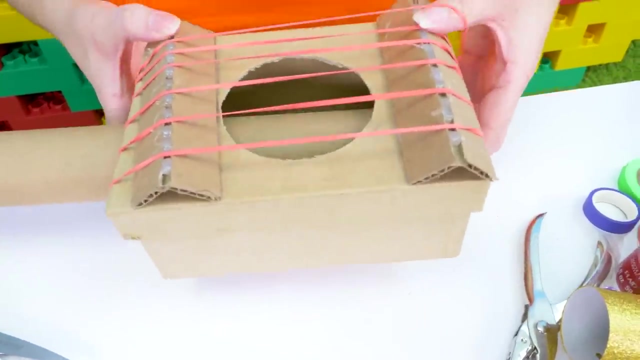 And now I think we're just ready for the strings. All we have to do is put the strings on the guitar very carefully, Make sure we don't pop any. There's five and our final string, string number six. You want to see how it plays? 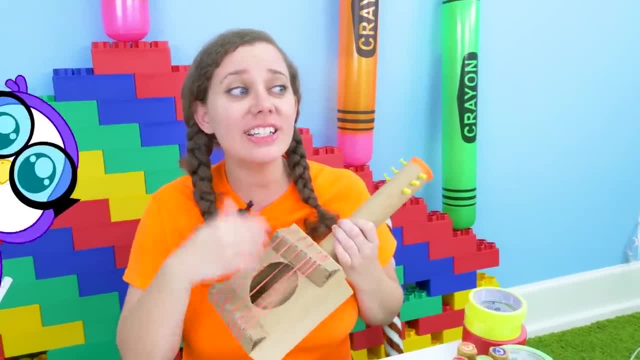 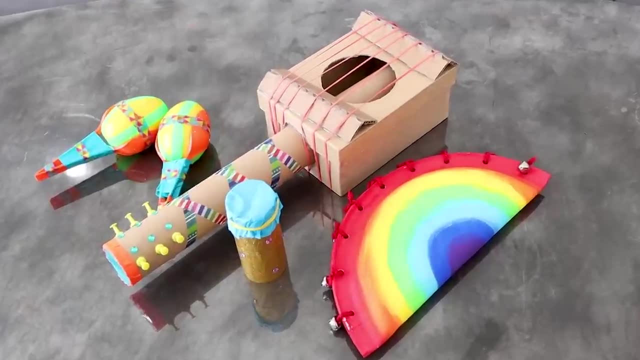 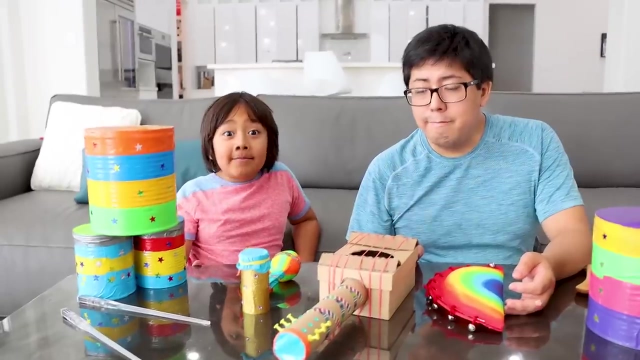 You recognize that song right. Twinkle, twinkle little star. How I wonder, Whoa? Thank you so much, Peck. Those are so cool. I'm going to test them out. I'm going to test out this guitar. 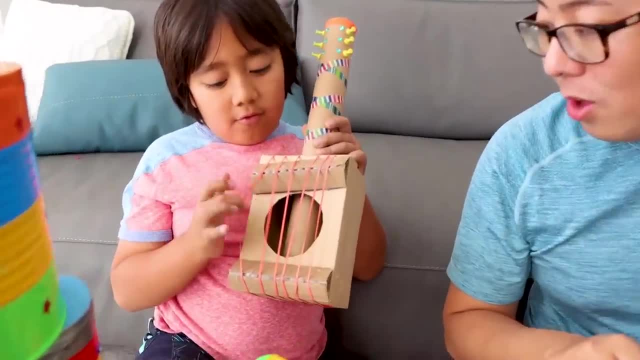 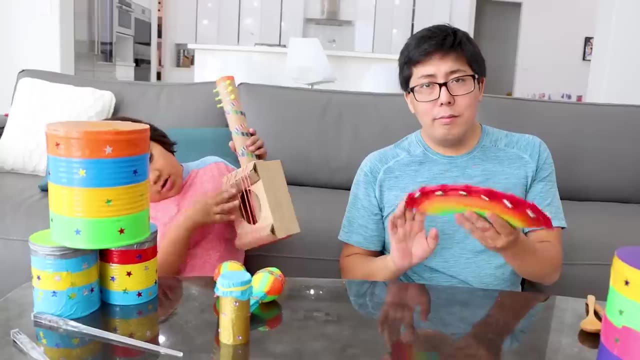 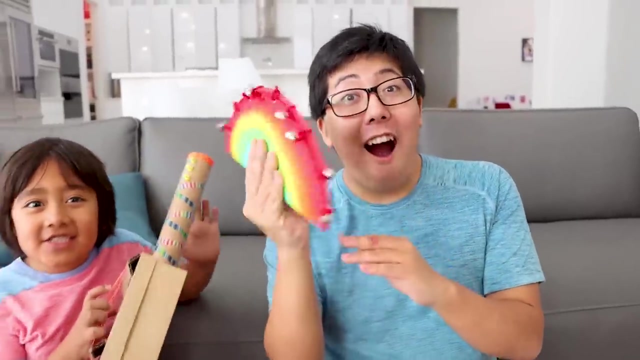 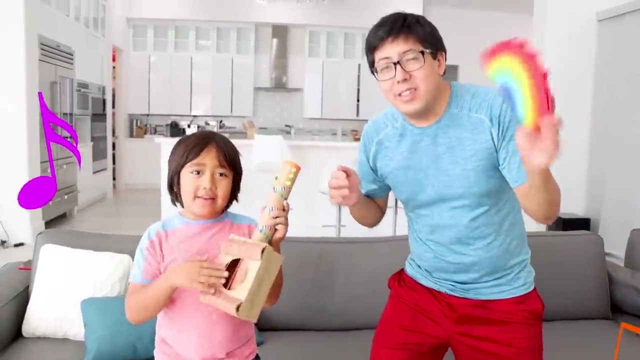 Whoa cool Does it make a sound? Yeah, they all make different sounds. Whoa, look, Ryan, This tambourine also make a noise. Whoa, Let's jam. Happy birthday to you. Happy birthday to you. 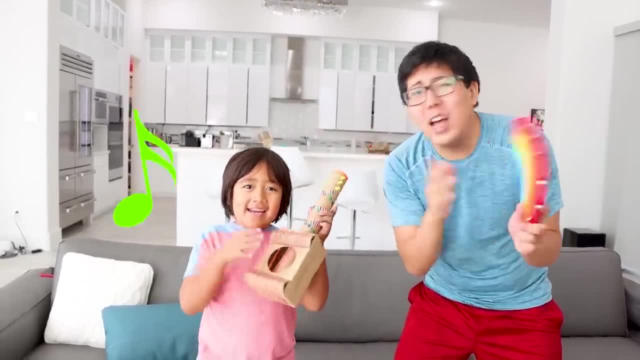 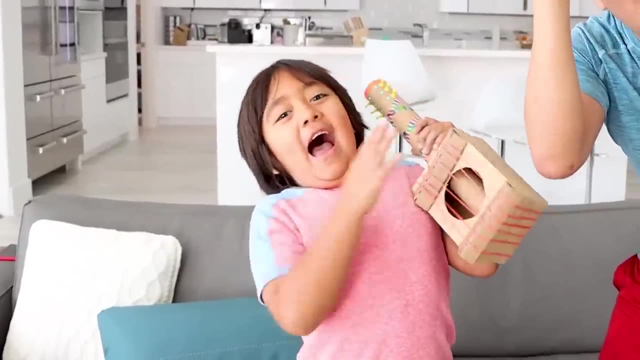 Happy birthday, dear somebody, Somebody out there. Happy birthday to you. Whoo Wah wah. I have two hands, You do too. I have two hands, You do too. I have two hands, You do too. 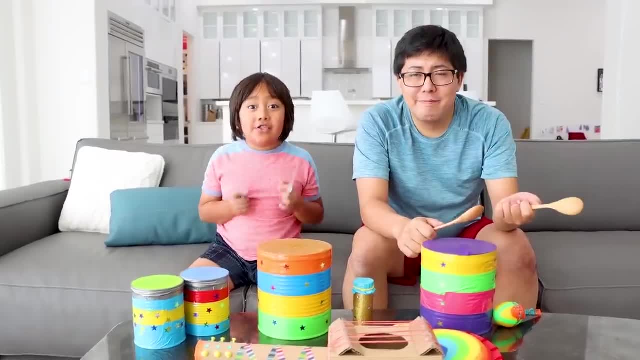 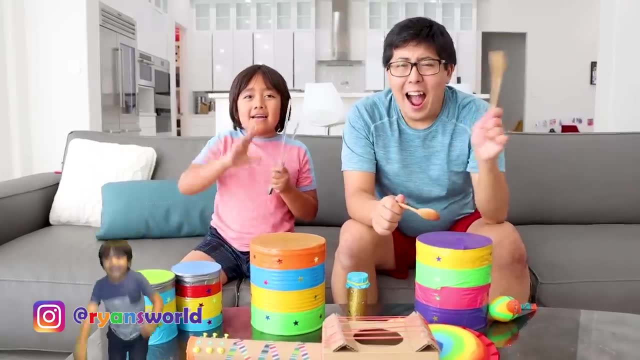 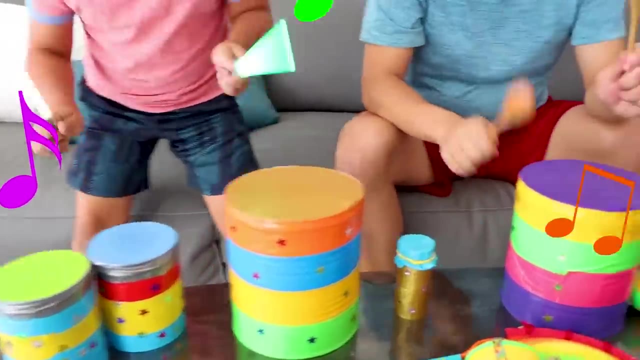 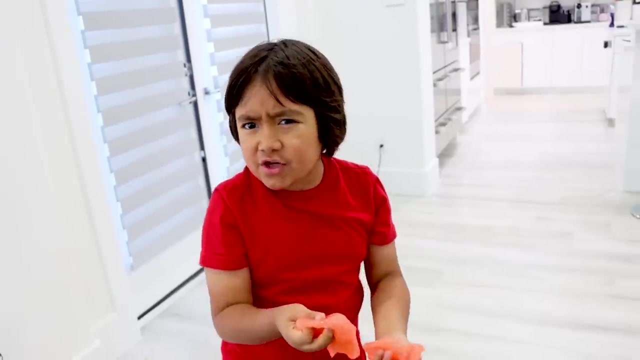 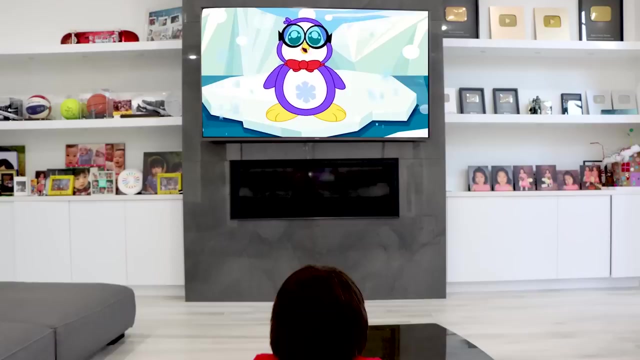 I have two hands. I forgot the rest. Thank you for watching our do it yourself instrument video And if you're at home, maybe you can try to make these too. Bye, Remember: always stay happy, Bye, bye. hey, Ryan, who's that? what is this? oops, sorry, Ryan, I left a glass of dirty. 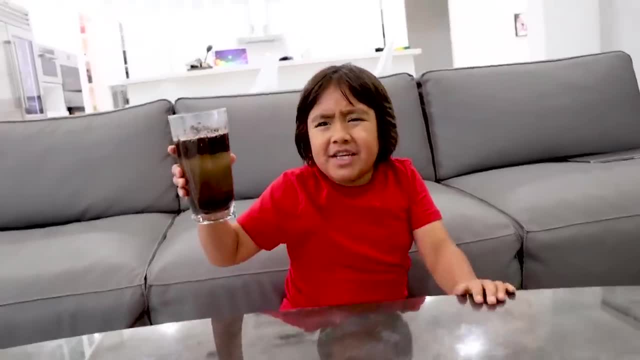 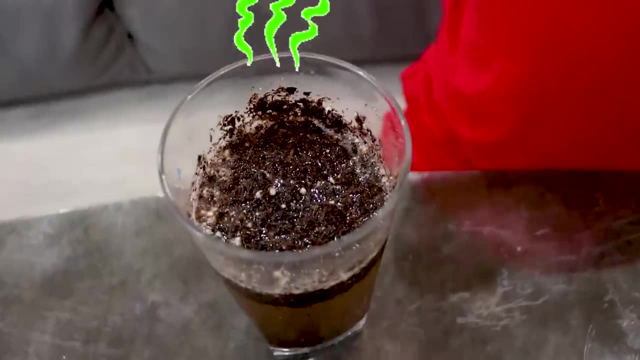 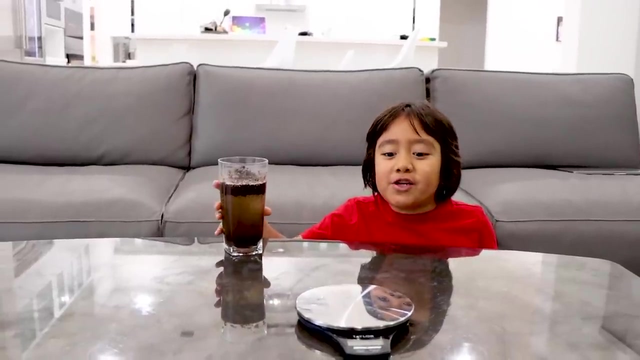 water there on accident. you know you cannot drink this. this is dirty heck. I have an idea: maybe there's a way to filter out all the dirty stuff. send it to the lab, Ryan, you know. find a way to get the dirt out. I'm sending this water to you. Peck teleportation device. 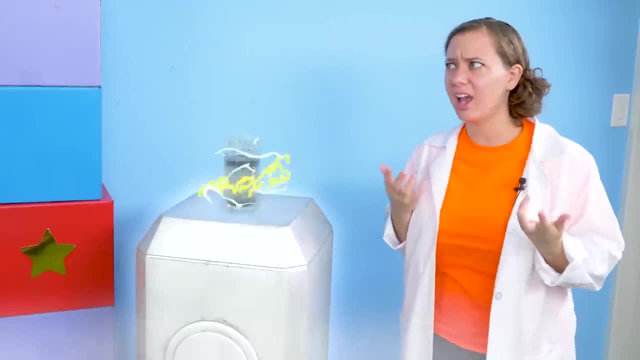 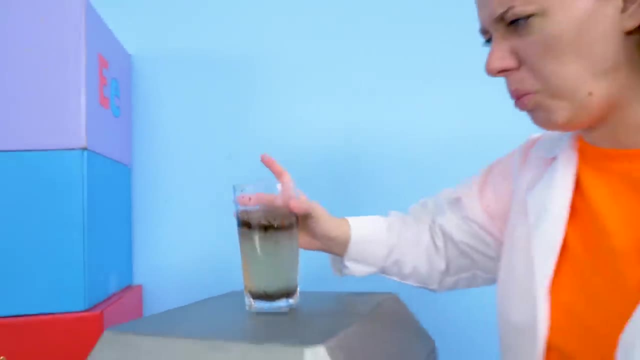 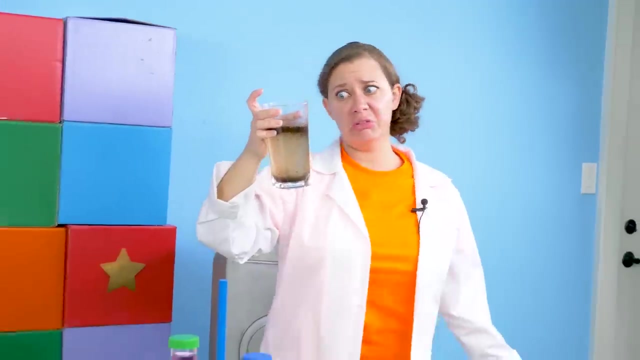 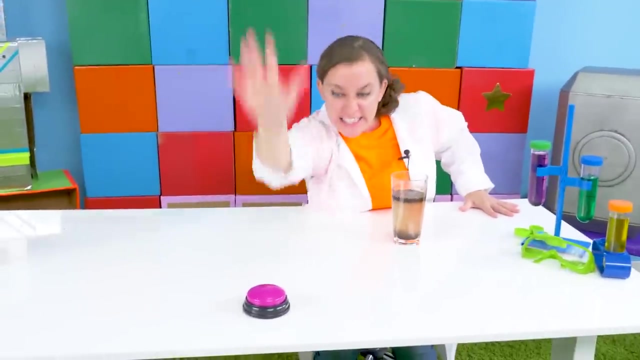 it looks like Ryan is sending us another science experiment. I wonder what this one could be. hmm, wait a second. is that water? it's really dirty water. we can't do anything with this. uh, we really need to clean this water up. hmm, I know just who to call for help. we need Peck. 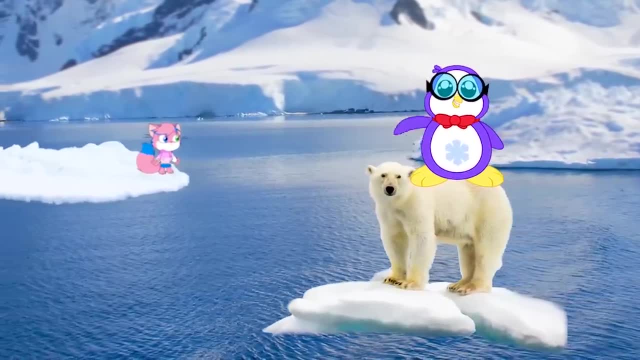 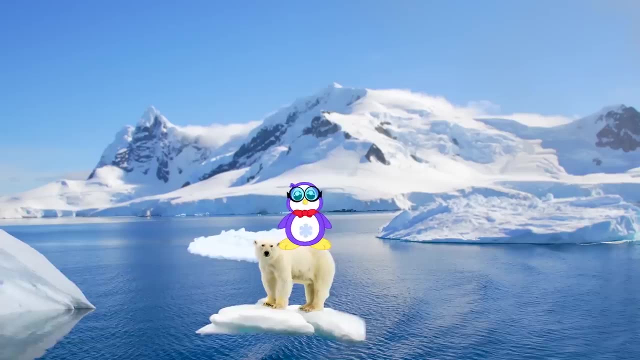 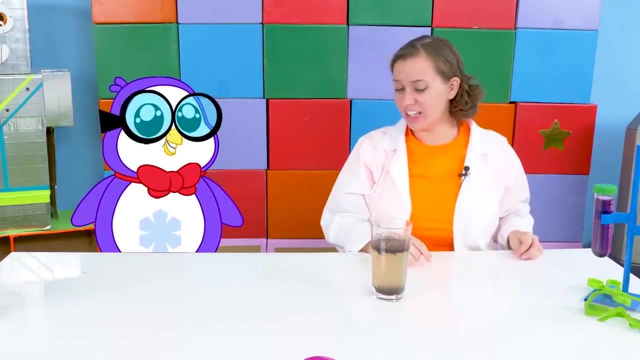 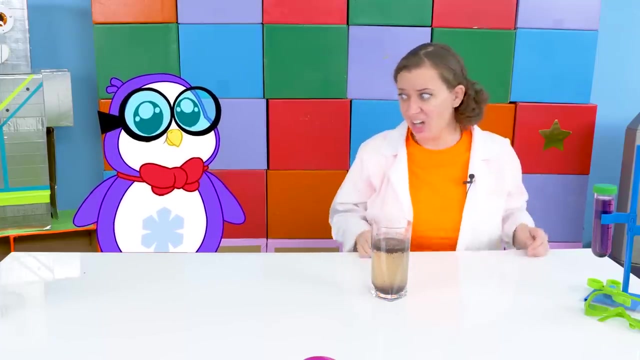 head this way for another 8000 thousand miles and you should make it to the North Pole. huh, looks like I'm needed in the lab later, buddy, what's today's science experiment? well, Ryan sent us this glass of water, but it is really dirty, so I think we need to somehow clean it up. I think we should. 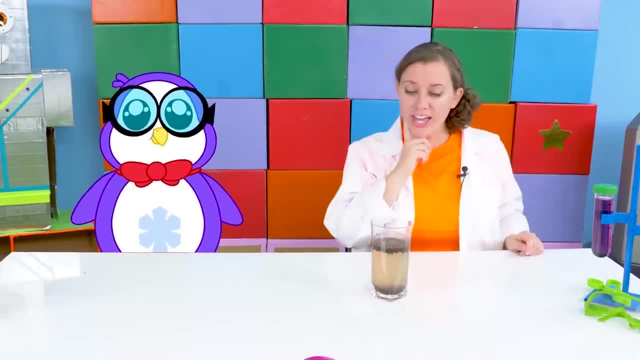 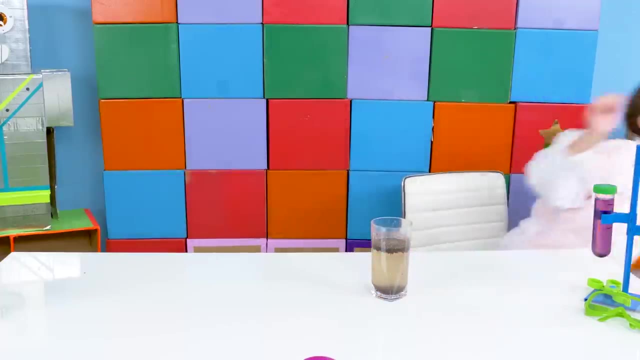 make a filter to get rid of the dirt. oh, that is a great idea, but how are we gonna? I think we can use everyday household items. oh, I think I know some stuff that we could use me too. let's get to it, let's go. hmm, something to use as a 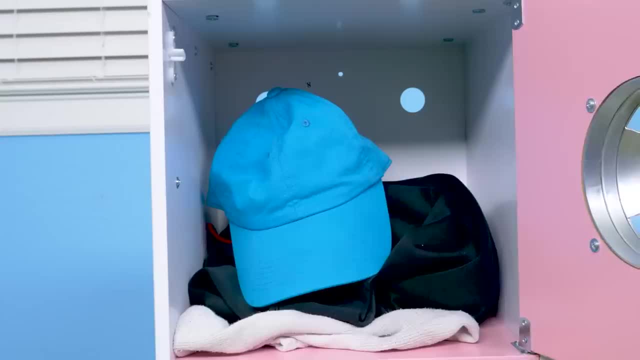 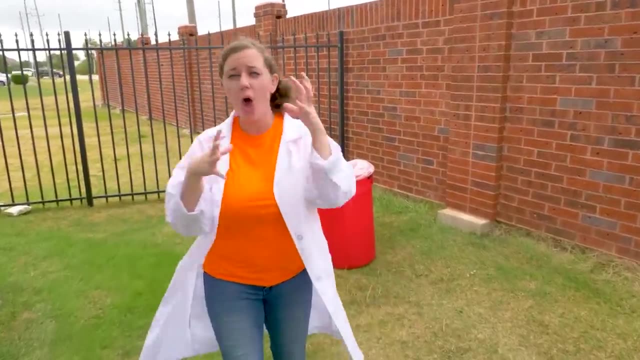 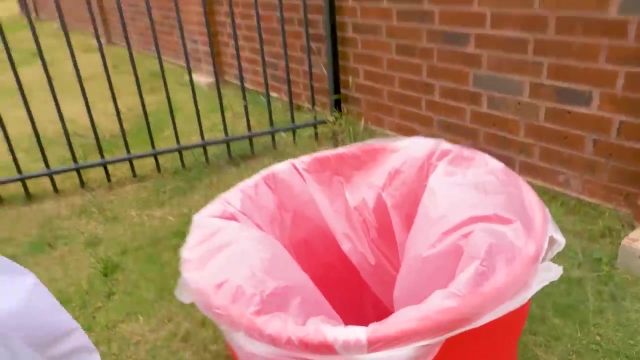 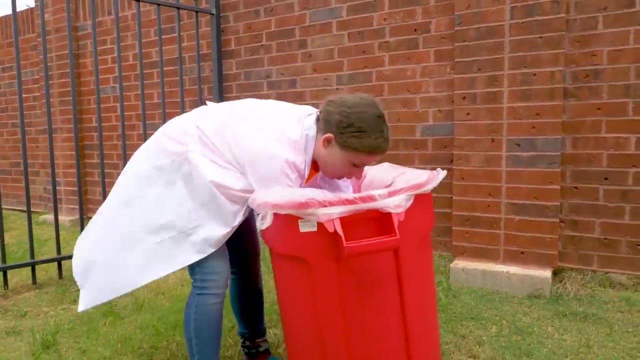 filter, maybe something in the dryer? let's see. oh, here we go, the sock. so we really need to find something that we can put all of our things in and something to hold it all together, but I don't know what. do you guys see anything? oh, of course, there's probably something in here. let's check. oh, my goodness, this. 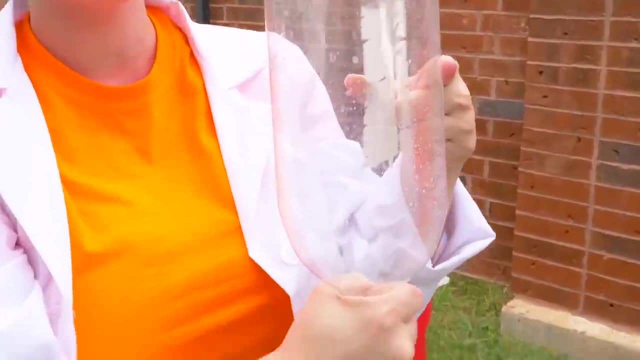 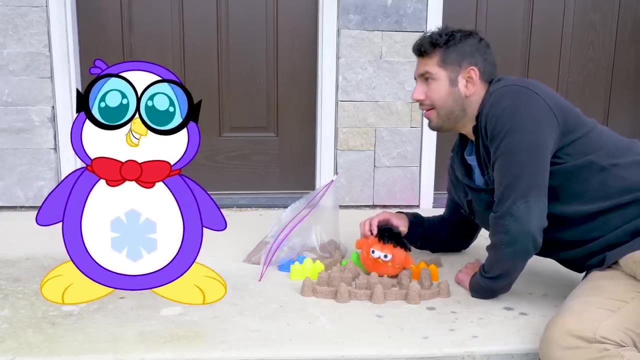 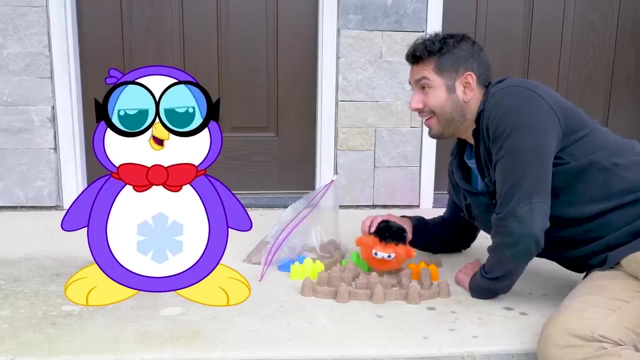 is perfect. it's gonna work great. oh hey, Daniel, is it sand you're playing with? oh hey, peg. yeah, I'm making some sand castles. you want to play with me? um no, I'm actually here to play with you. oh hey, Daniel, is it sand you're playing with? oh hey, peg, yeah, I'm making some sand castles. you want to play with me? oh no, I'm actually here. 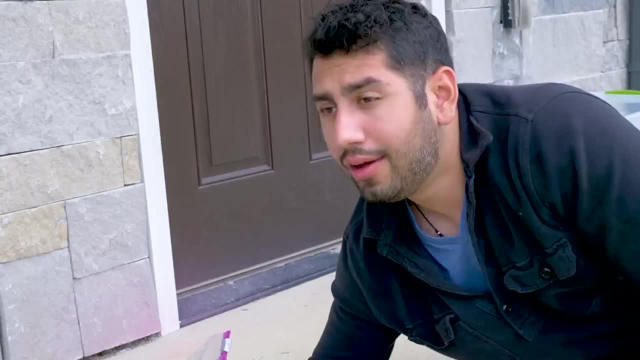 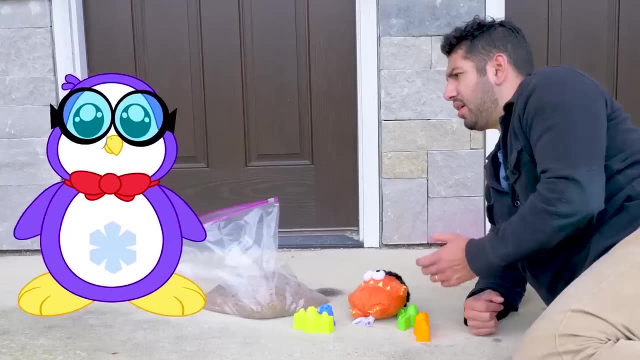 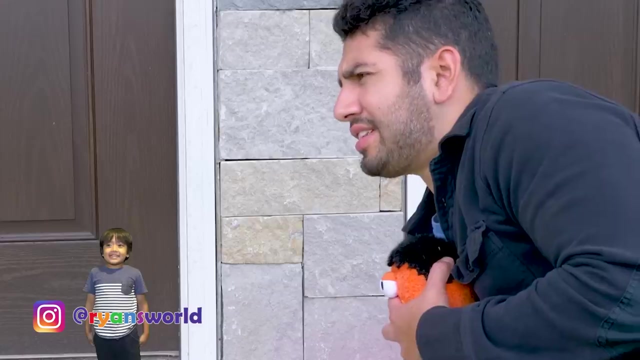 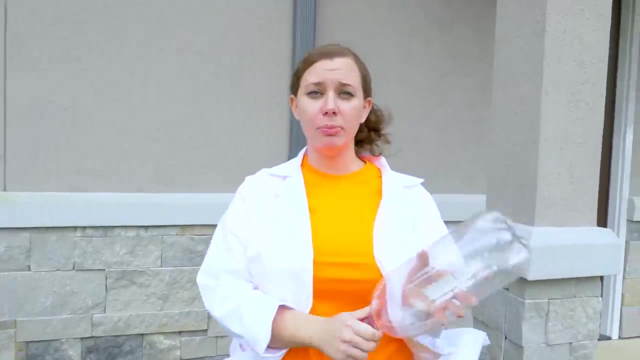 doing a science experiment. but I could use the sand. yeah, of course here, take some gee. thanks, Daniel, don't mind if I do. thanks for your contribution to science. oh, okay, fine, I guess take it all. I mean, I wasn't using it or anything, so I got my bottle, but we need things to build the actual filter. so what can we use? what can we actually use? 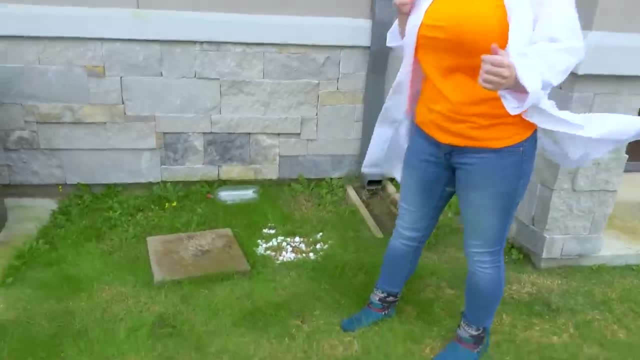 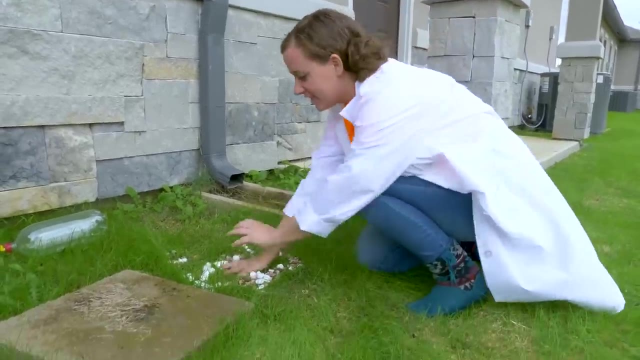 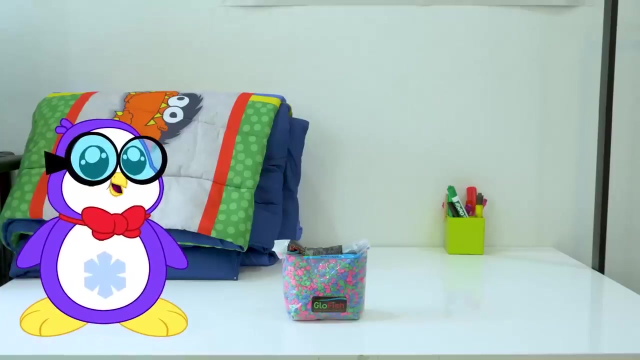 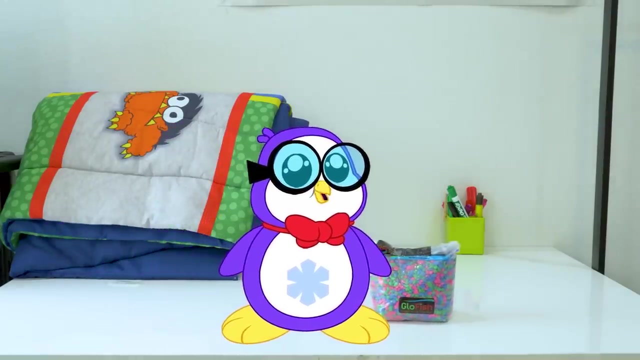 what can we actually use? I got it. we can use these rocks. they're perfect. there's so many of them, man, this is gonna work so good. ooh, a shiny bag of fish gravel. I can totally use this to help filter out the dirt too. here we go. hmm well, we're in the kitchen right now. 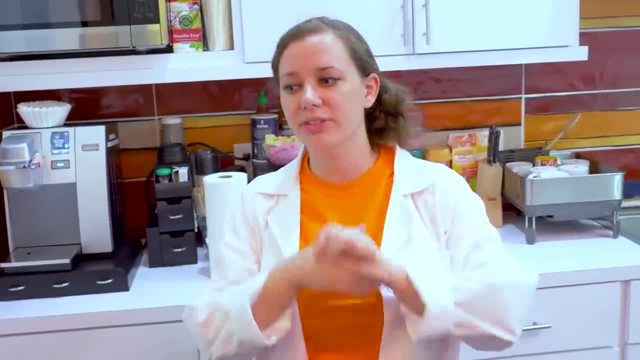 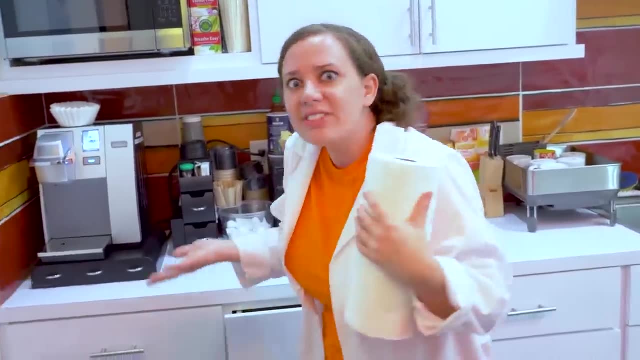 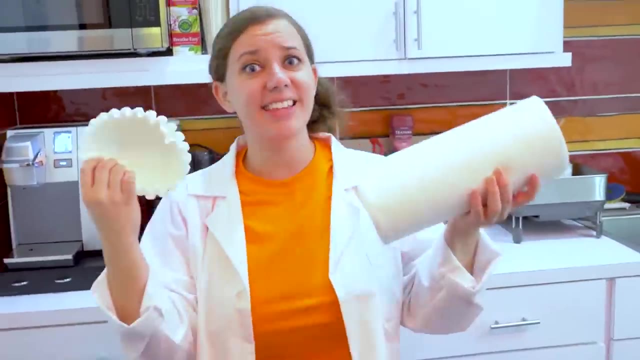 and there's got to be really good stuff that we can use this filter. so let's see. hmm, of course, paper towels that should work pretty good. wonder if there's anything else. coffee filters: I think these items are great, but let's see what Peg's got we. 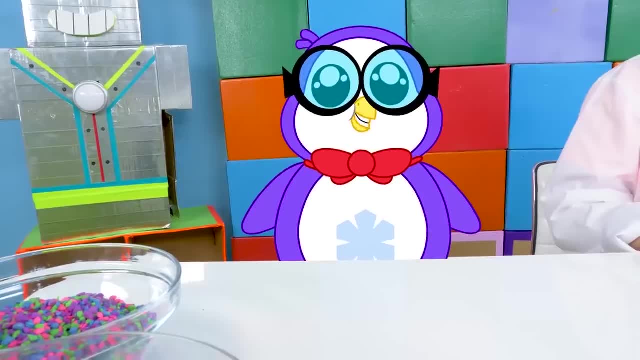 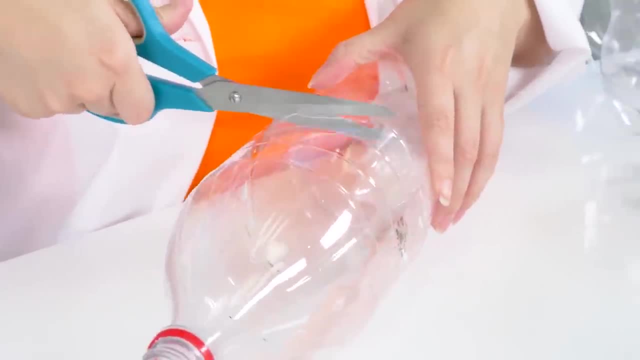 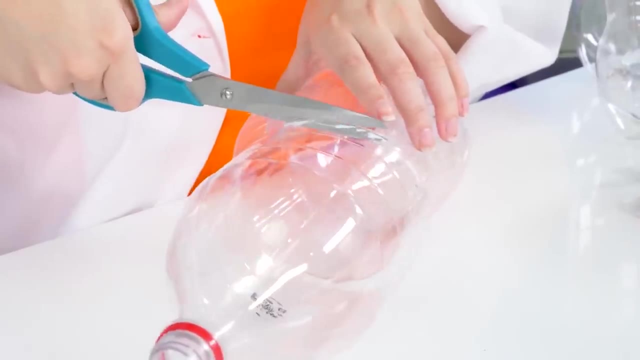 gather all the needed materials and an adult. what do we do now? so the first thing we need to do is to make the outside of our container for our filter by cutting up this water bottle. ooh, that's looking so good. there we go. it's perfect. now the really cool part. 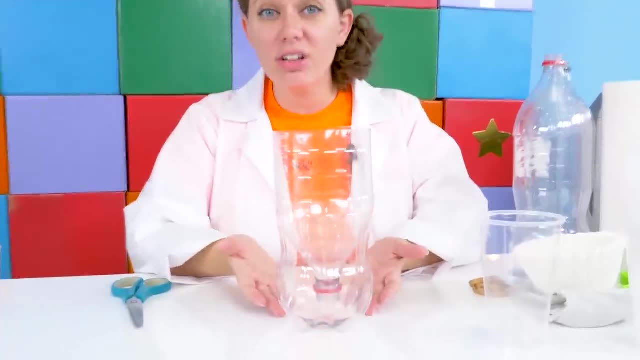 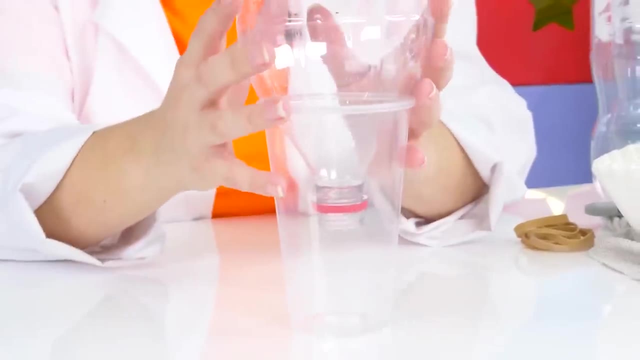 about using a bottle is we could use the bottom part to catch all of our water, but I found this cup here. I really like it because of how tall it is and I think we're gonna be able to see our results really well in this. oh, I see now that we 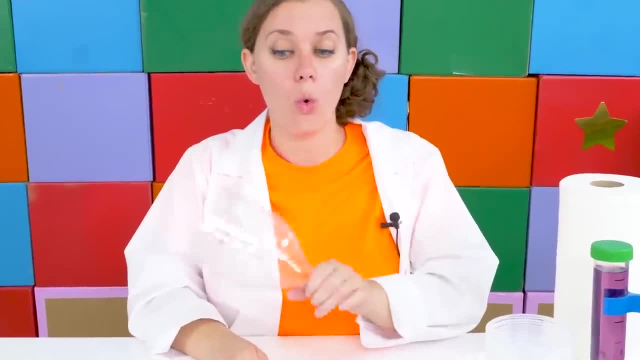 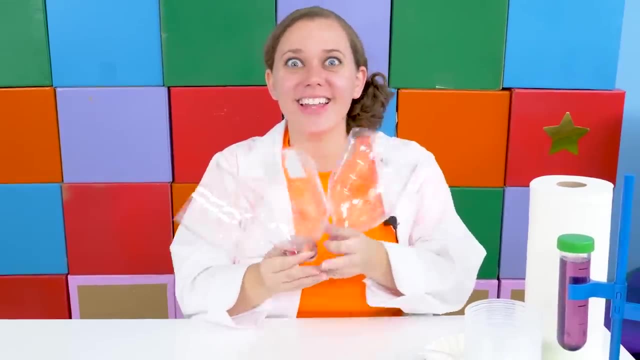 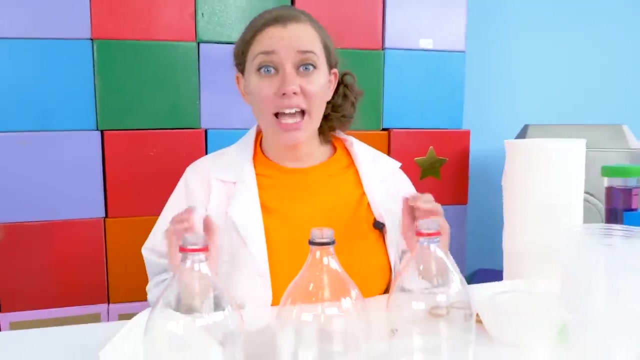 finished our first bottle. all we need is two and three bottles. That is perfect for our experiment. Let's get started. How did you do that? I must be seeing things Alright. now we're going to start with our three different filter bases. 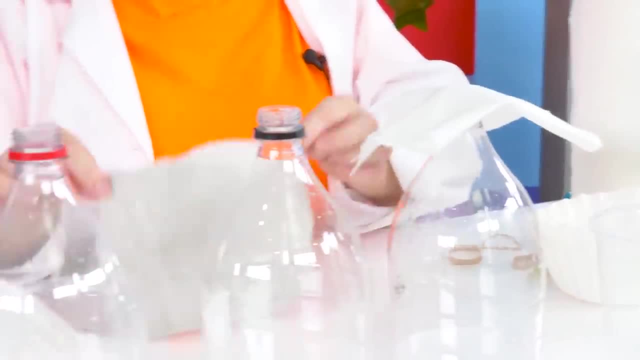 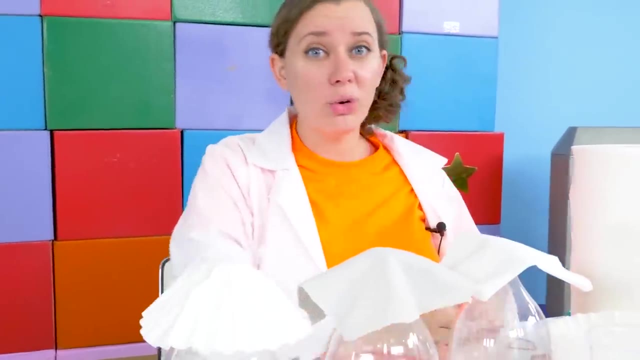 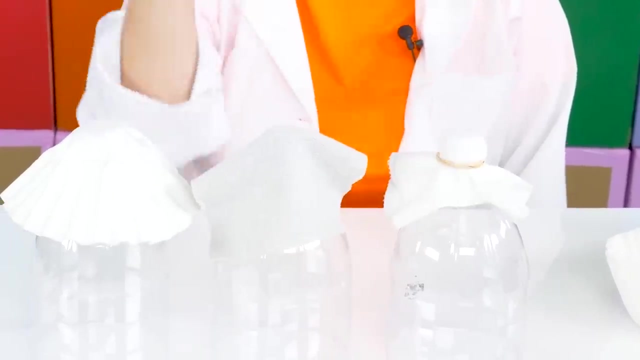 So paper towels is our first one, This dirty old sock is number two, And coffee filters is our third one. We can hold them into place with these really strong rubber bands. Okay, rubber bands one, two, three, Nice and secure. 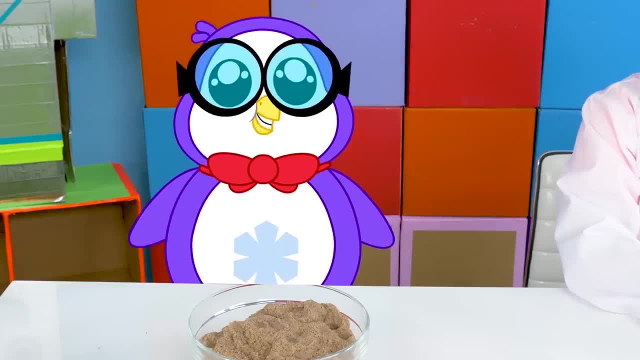 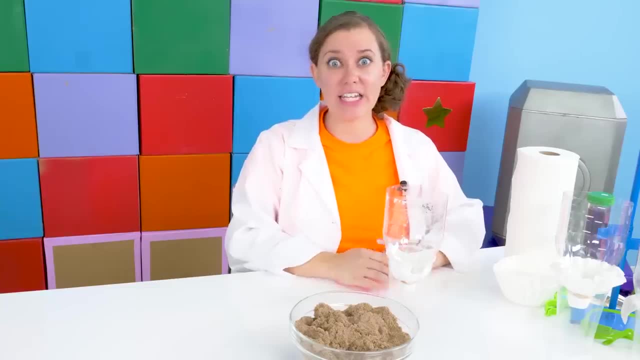 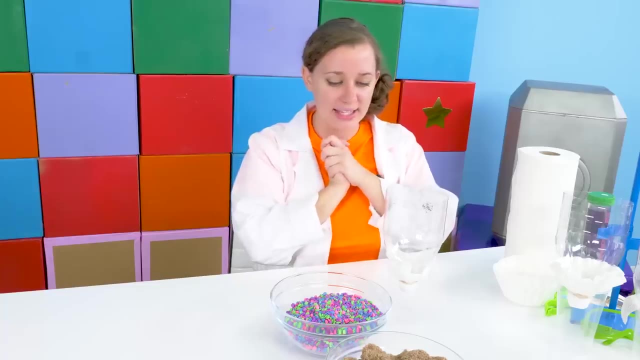 Hey, Peck, could you pass me the sand? One bowl of sand coming right up, Whoa, that looks like fun. Next, we need gravel. Here's some gravelly gravel. Last thing that we need is rocks, Big rocks. 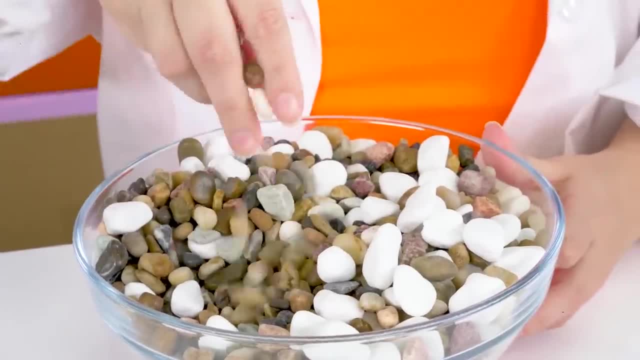 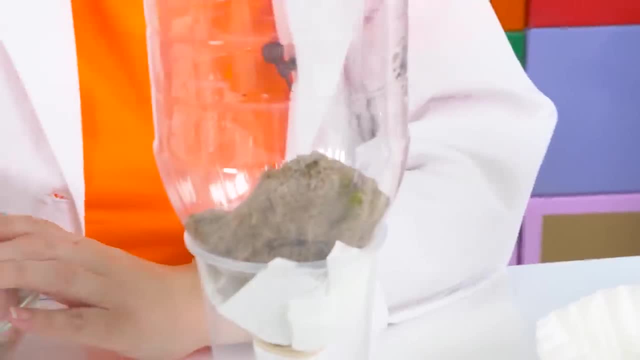 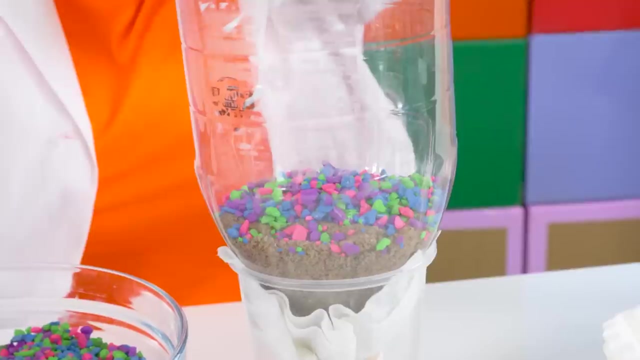 Whoa, that's perfect. Alright, starting with the sand, We have to make sure it goes all the way down to the bottom. This kinetic sand is nice. It doesn't get messy. Next up is the gravel. This is going to be so pretty. I love the colors. 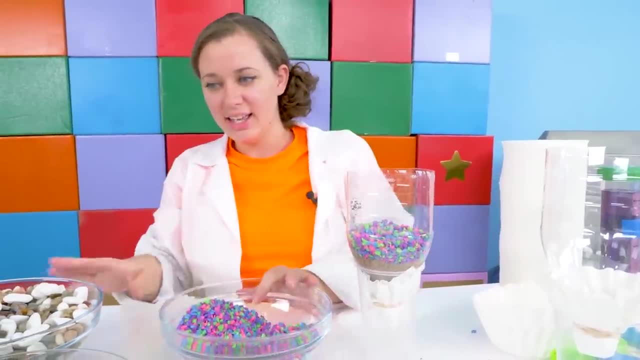 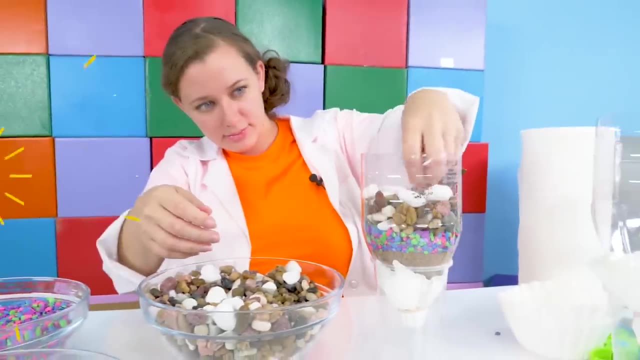 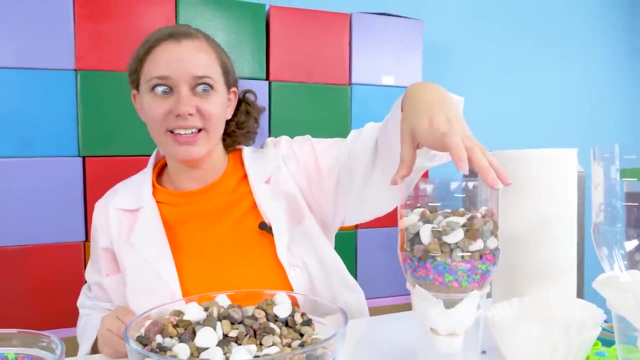 I think that looks pretty Pretty good. So now we need these big heavy rocks Looking good. Hey, can I borrow one of those pebbles later? There you go. That looks pretty good Now that we have our first one built all the way. we just have to do the same for two and three. 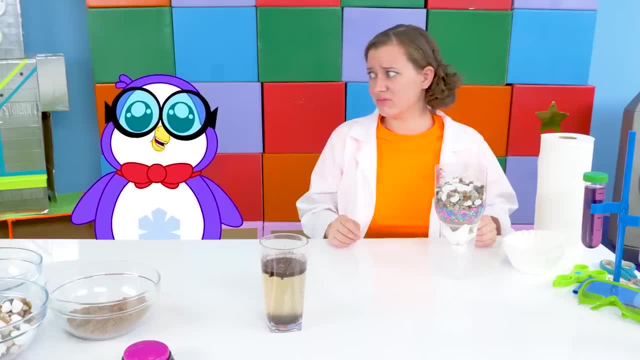 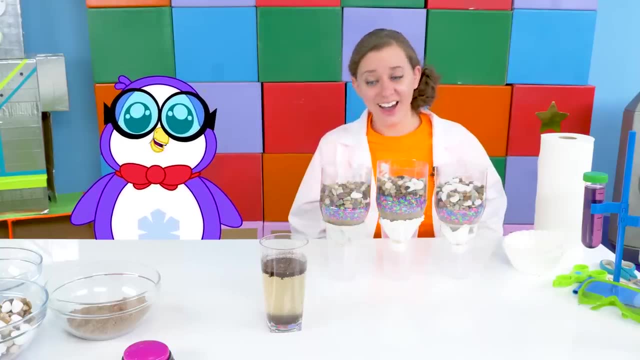 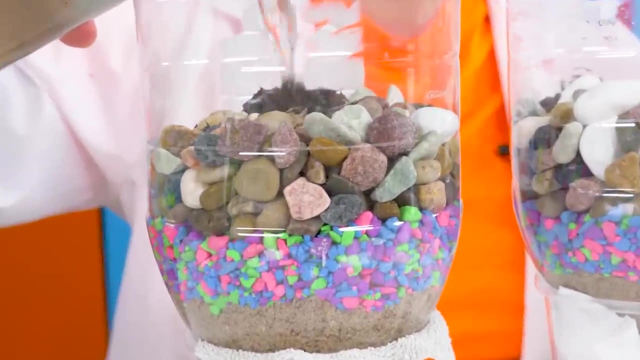 Oh, I can use my special blaster to get the job done. Pew Whoa, that is incredible. Aw shucks, It was nothing. Okay, here's a moment of truth. Let's see if our filters work. I can see the water filling up and the little pieces of dirt swimming around like fish. 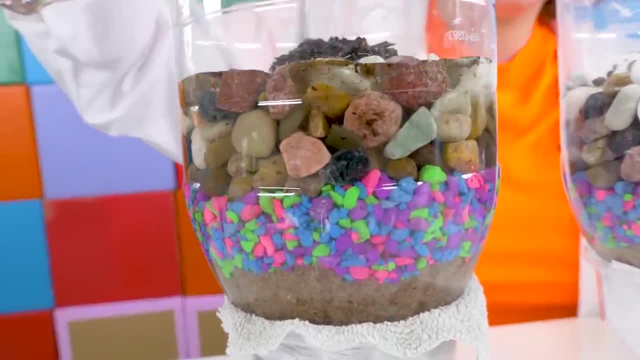 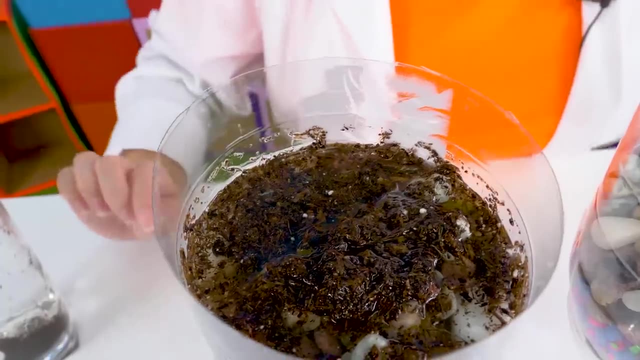 I'm getting a little hungry now. We're already starting to get some water coming out. Whoa, look at that. It looks like a lot of the dirt is getting caught by these rocks, and maybe some of the smaller dirt by these smaller rocks. 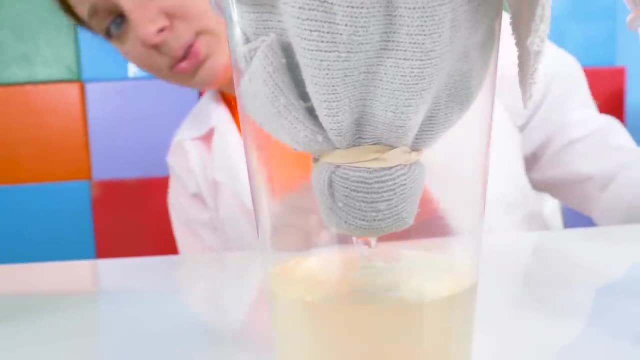 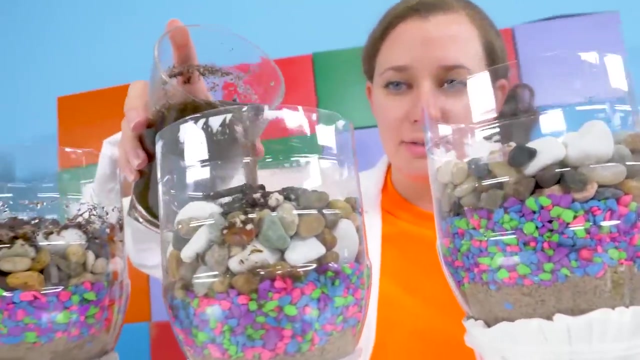 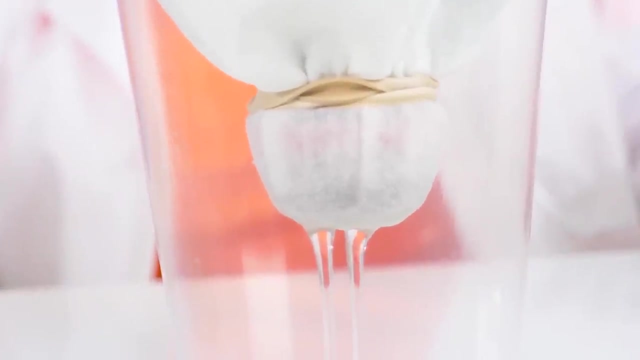 The sand looks like it's doing a lot of work too. Four times speed, Whoa. All right, let's see how the paper towel does Whoa. That rubber band sure is doing its job. And the last one is the coffee filter. 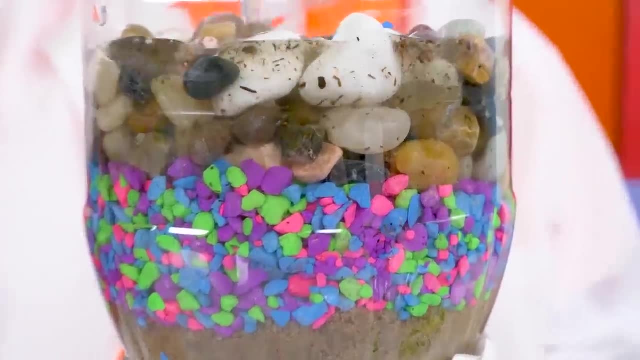 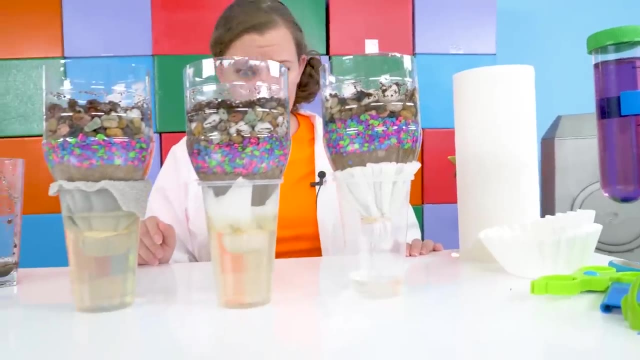 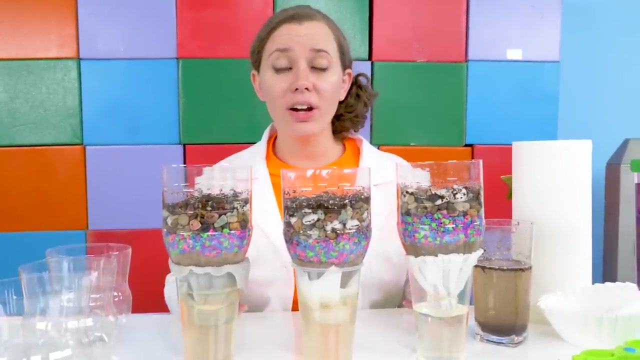 I mean, it is a filter on the end of a filter, Whoa. So this one looks like it's already coming out more clear than the other two. Brilliant deduction Bree. Now that we have all of our water filtered, let's take a look. 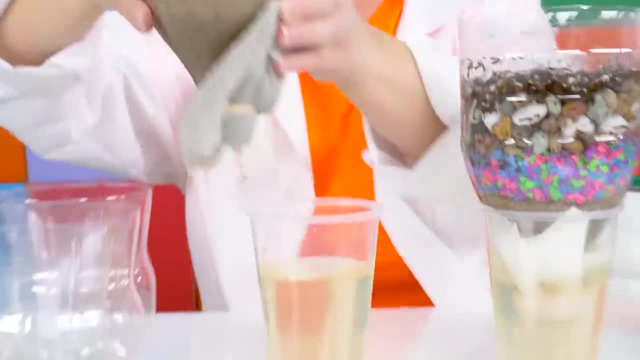 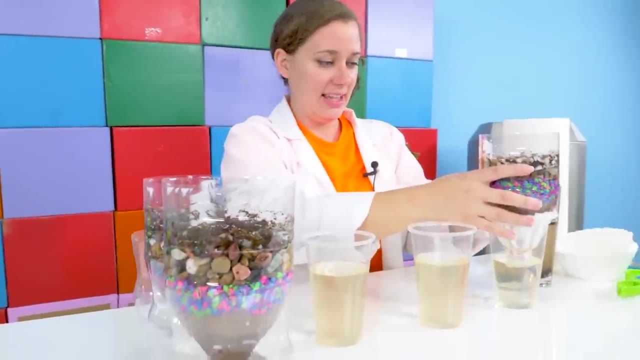 Let's compare them. Okay, so we're just going to take these guys out and put them in here. Oh gosh, be careful. Ooh, There we go. And last but not least, the coffee filter. Yay. 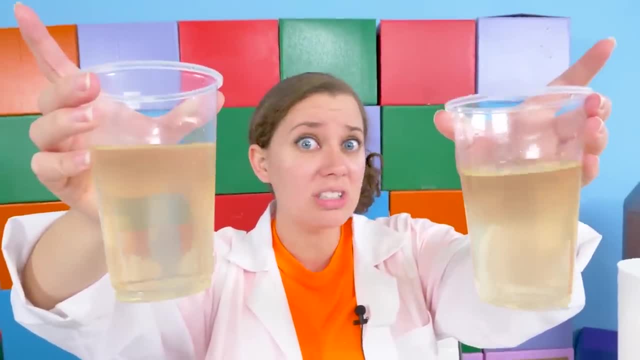 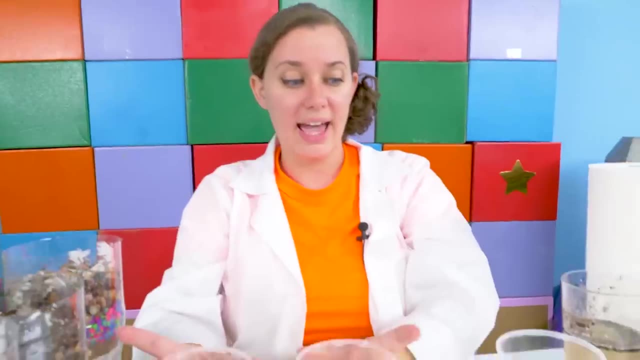 Well, these two, I don't think they did as well. It worked a lot. There's obviously no dirt in there, but they look pretty cloudy and I can't really see through them that. well, Now the coffee filter: Whoa. 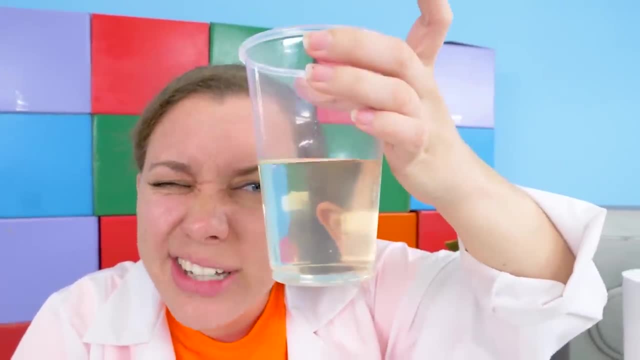 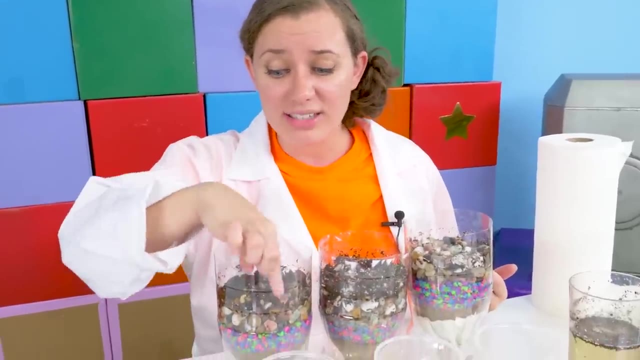 That is so clear. Look at that, I can see straight through it. It's time to review the results for Ryan. Okay, so I think the results show us that the rocks and the gravel and the sand do a really good job of getting all the dirt out. 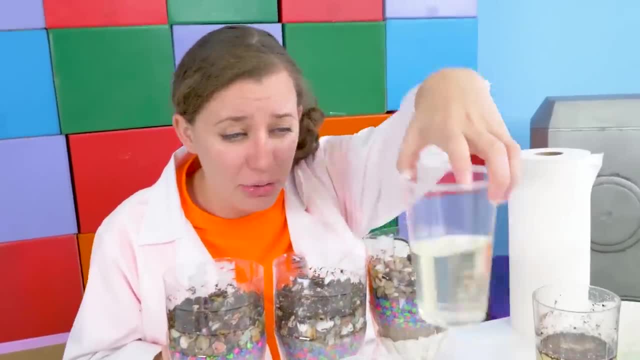 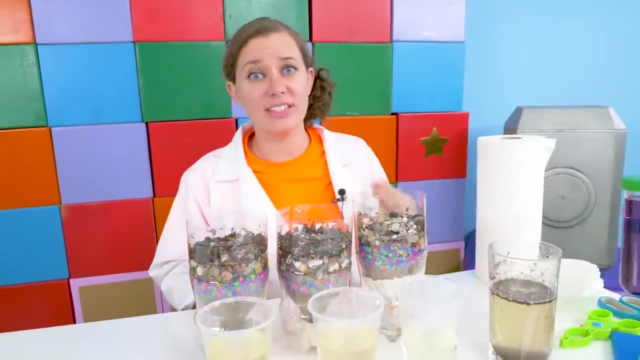 but the coffee filter is the only one that can get all those little teeny tiny parts out, which makes it clear like that. I think it's safe to say the coffee filter definitely did the best, But it does look better. Back to you, Ryan.